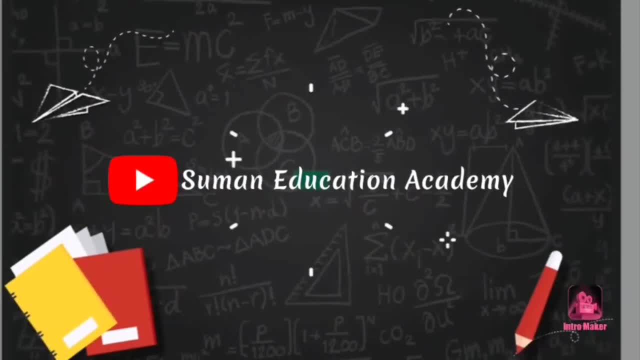 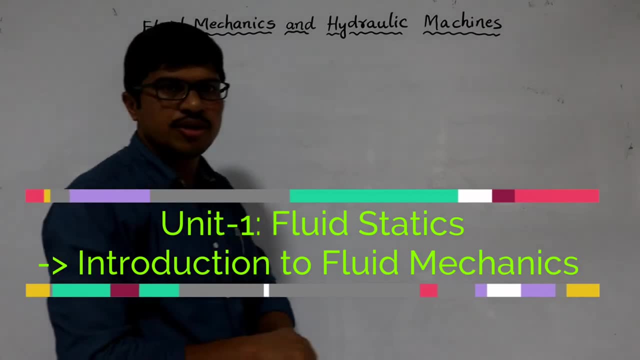 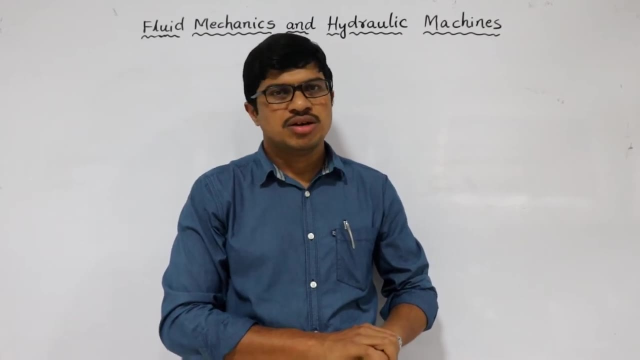 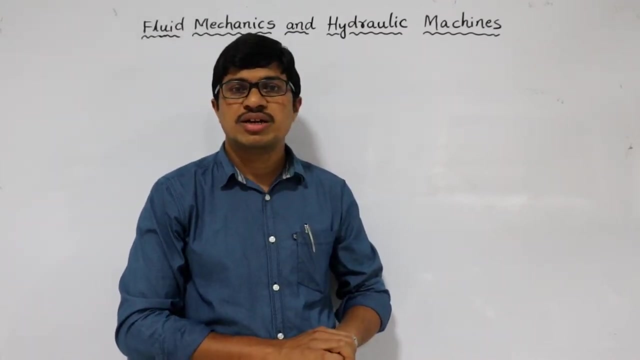 Hello everyone. this is Mr Suman. Welcome to Suman Education Academy. Hope you all are doing well In today's class I will continue. fluid mechanics and hydraulic machines- one of the very, very important subjects for mechanical and civil engineering students, not only for 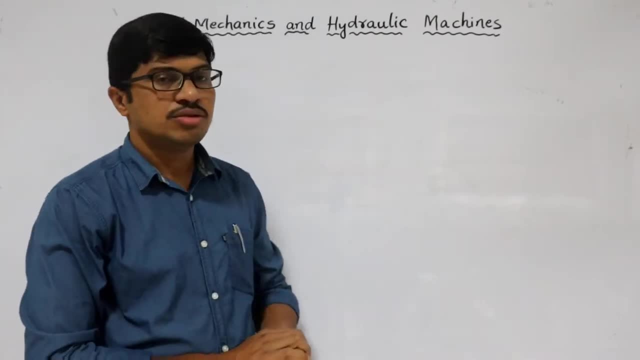 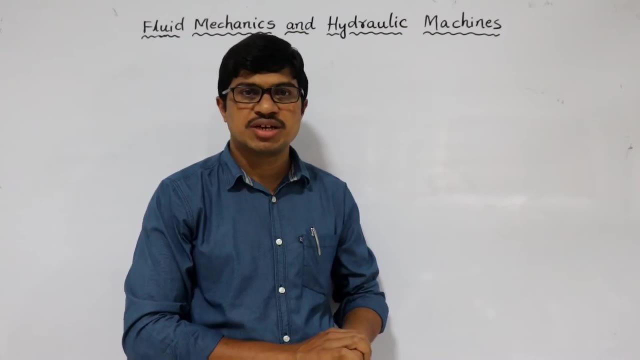 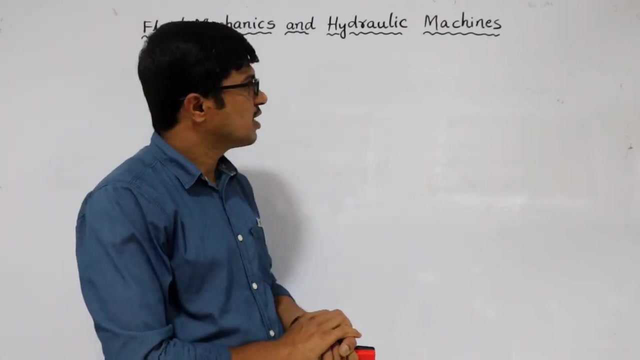 engineering. for diploma also- And this subject will help you for cracking the PS Genco and AP- Genco exams, which are conducted by the state government of Telangana, and AP, And for GATE also, you may expect 6 to 10 marks from fluid mechanics and hydraulic machines. 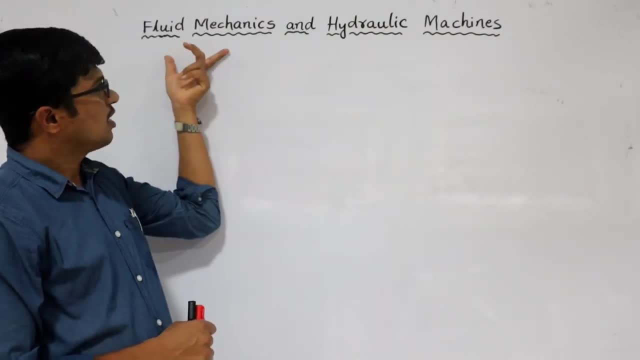 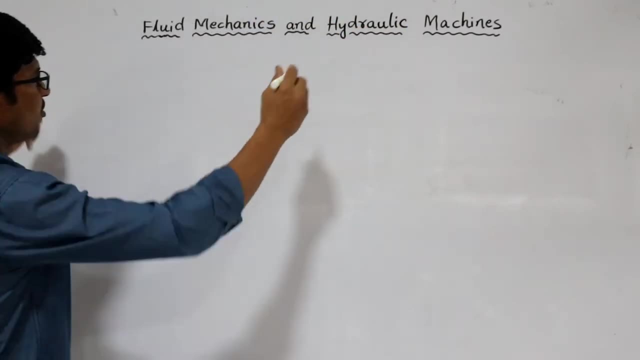 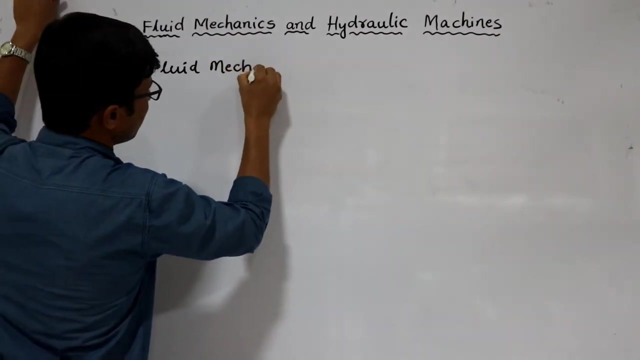 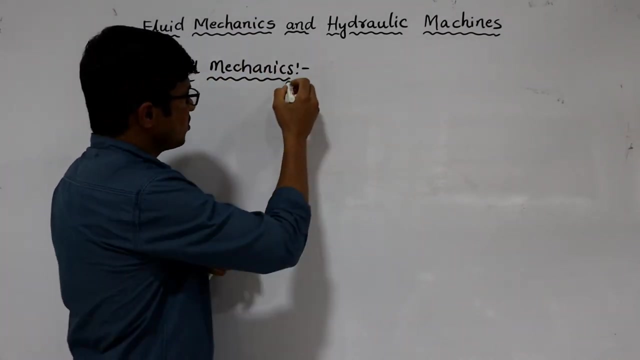 Right? So in today's class, let me continue fluid mechanics, And after completion of this, fluid mechanics, thereafter I will go for the hydraulic machines, Right? So let us continue fluid mechanics, now Fluid mechanics. So first, first of all, I think every one 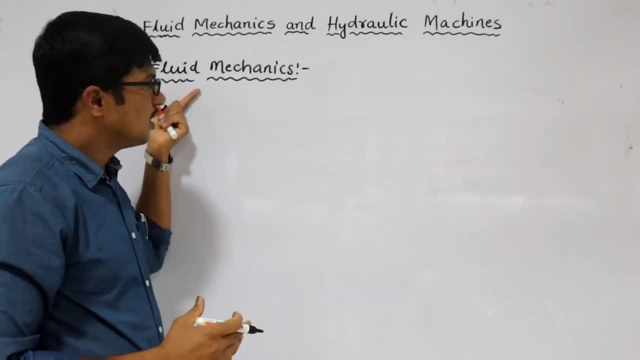 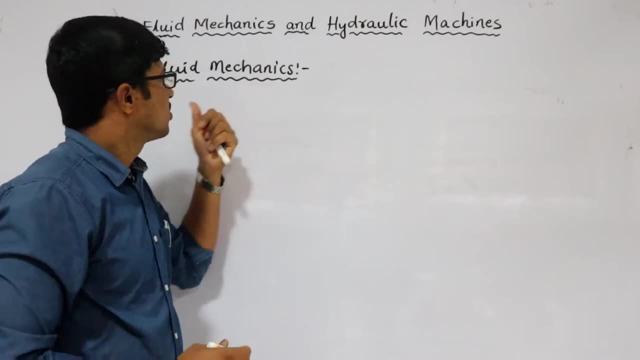 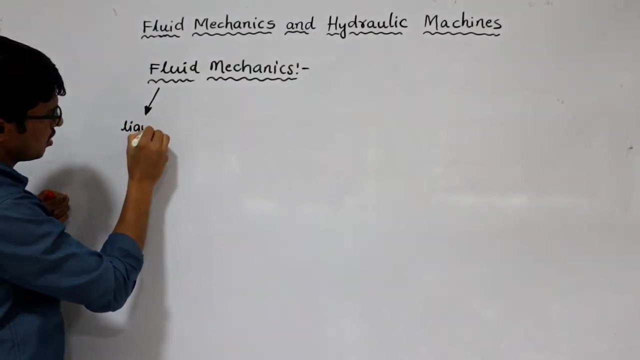 of you, everyone knows that. what is fluid? right, And what is? what do you mean by mechanics? So already you might have studied in engineering mechanics, right? So let us see here the first one Now: what is fluid? Fluid is fluid, is a fluid which is liquid. The fluid is. 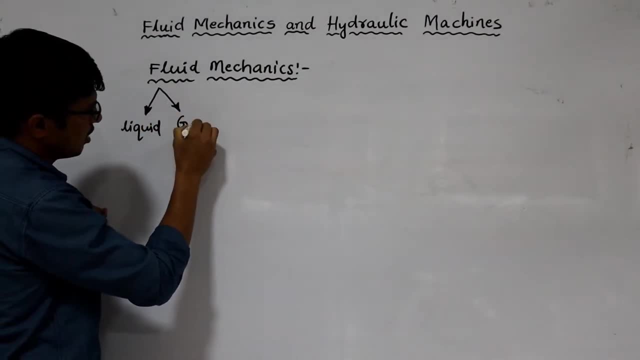 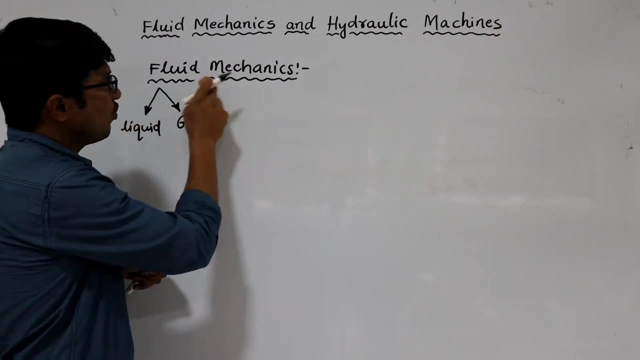 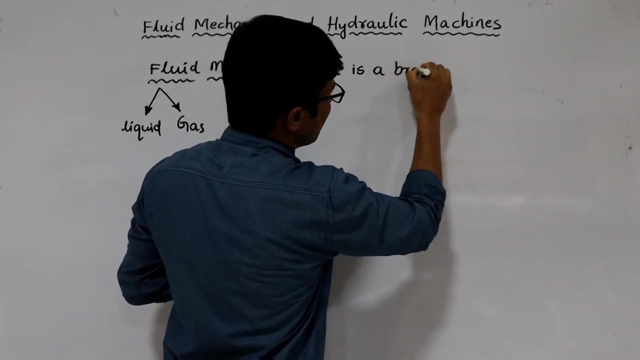 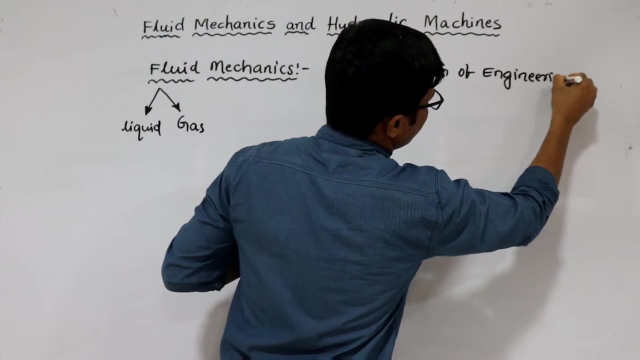 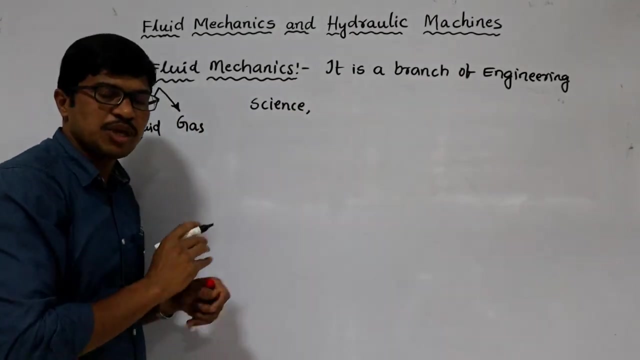 a liquid and gas. The fluid is a liquid or gas. And what is fluid mechanics then? The fluid mechanics? it is a, it is a branch of, branch of of a fluid. It is a branch of a Science, engineering science, branch of engineering science. sometimes we can write physical science also, right? 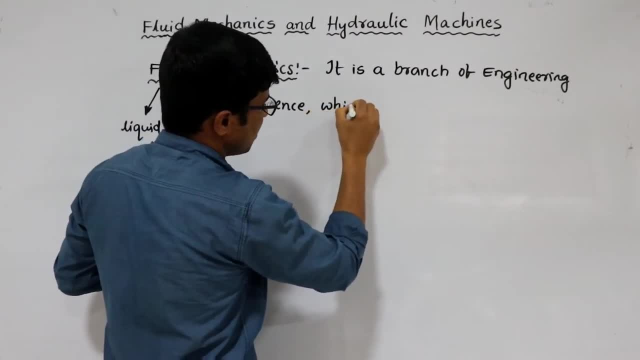 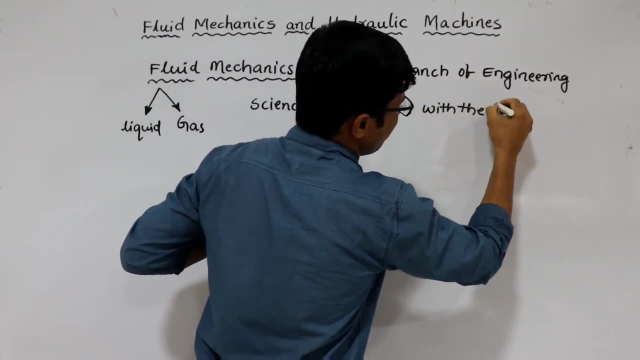 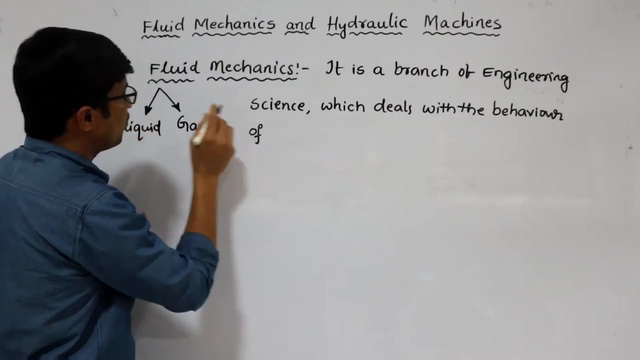 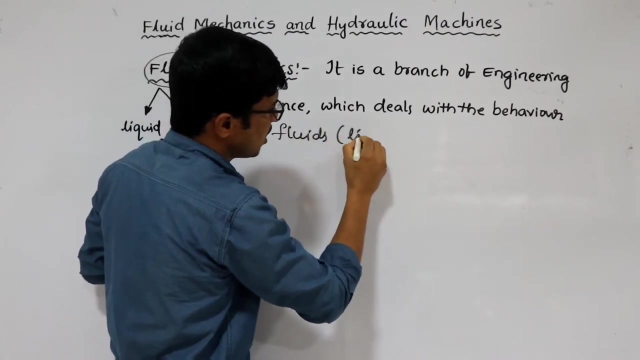 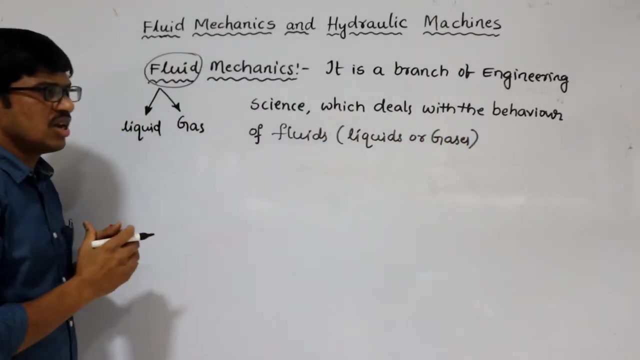 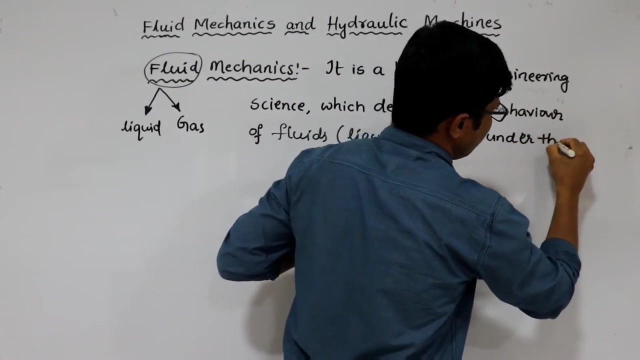 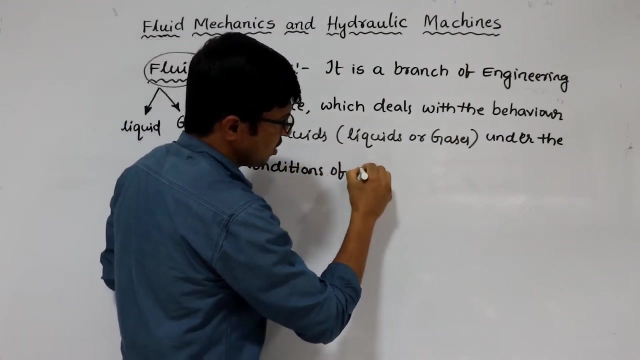 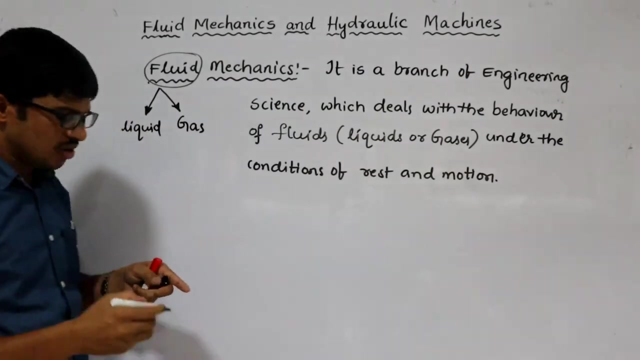 So which deals with the behavior, deals with the behavior of behavior of fluids, behavior of fluids. So these fluids are liquids or gases. These fluids are liquids or gases under under the conditions of, under the conditions of rest and motion, rest and motions, which is called fluid mechanics. 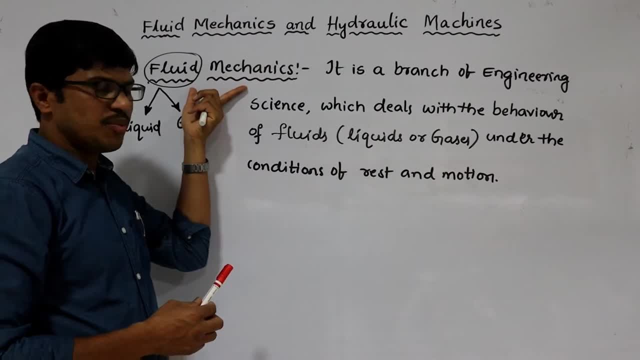 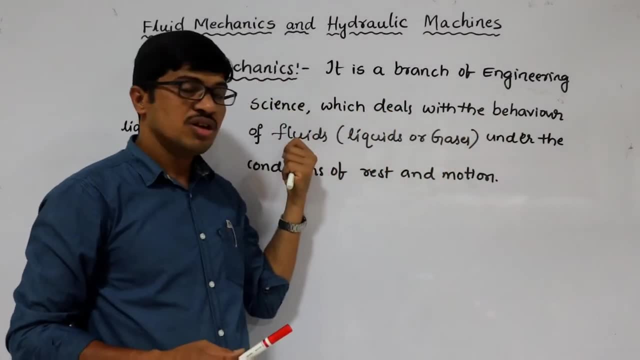 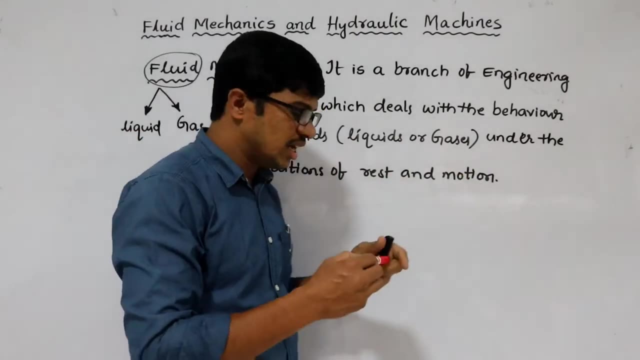 And it is also called mechanics of fluids. which is also called mechanics of fluids, So fluid mechanics. It is a branch of engineering science which deals with the behavior of fluids, which are liquid or gases, under the condition of rest and motion under the condition. 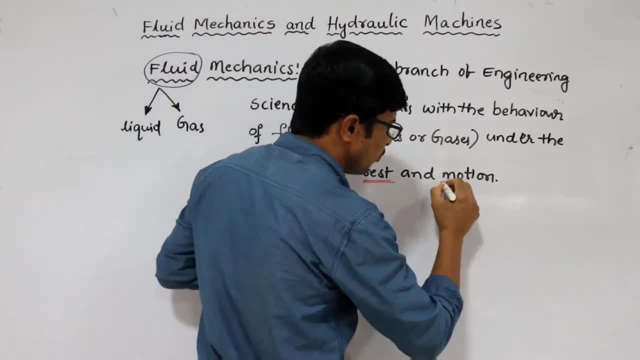 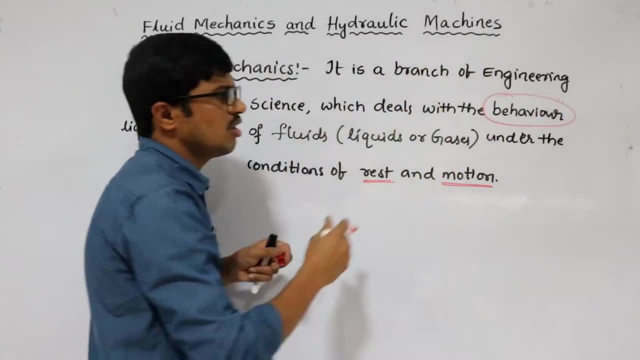 This is very important When the fluid is at rest and when the fluid which is in motion, and then where we need to find the behavior of the fluids, where we need to find the behavior of the fluids, that is called mechanism of the fluids right. 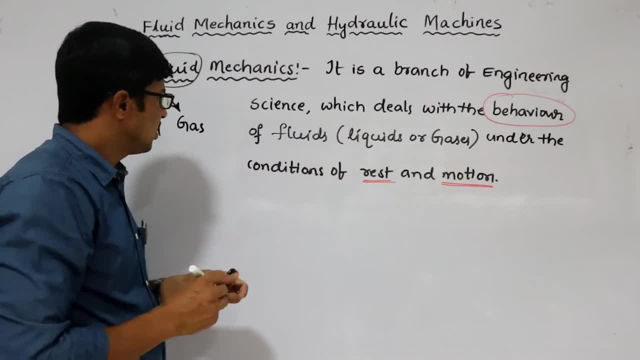 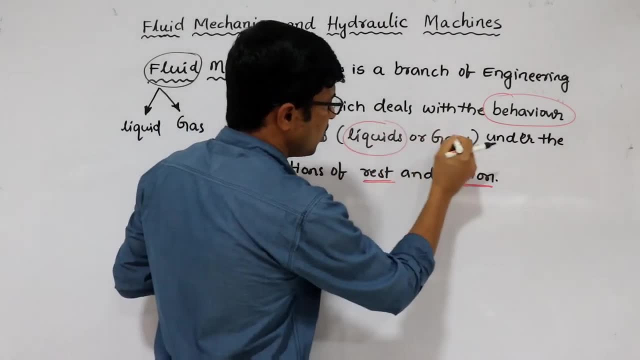 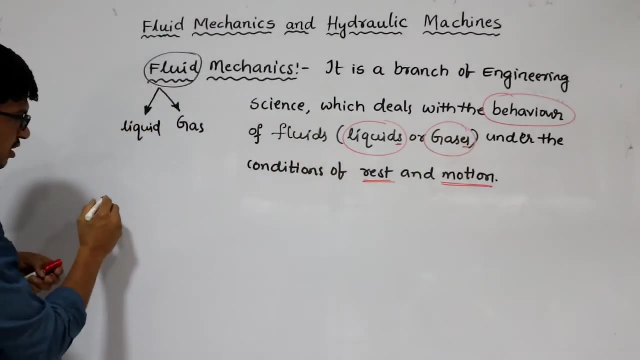 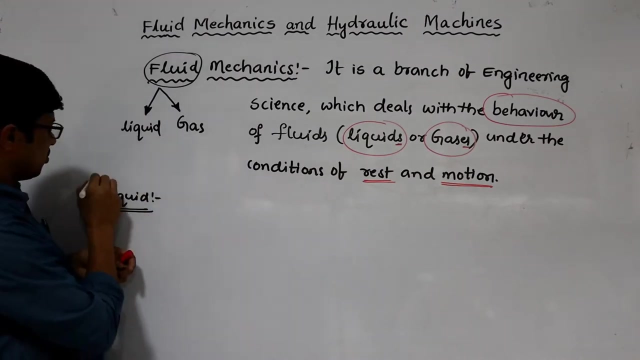 So this is called the fluid mechanics. Now next very important note: as I mentioned here the fluid, it may be liquids or gases. liquids or gases, So we have standard liquids. Let me consider here first liquid. So it is very important note that you should, you should have a minimum knowledge about the this particular note. 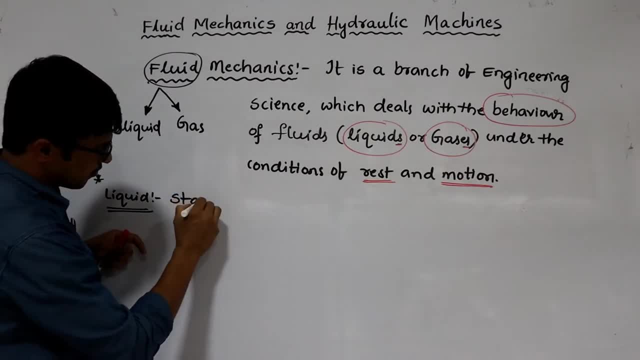 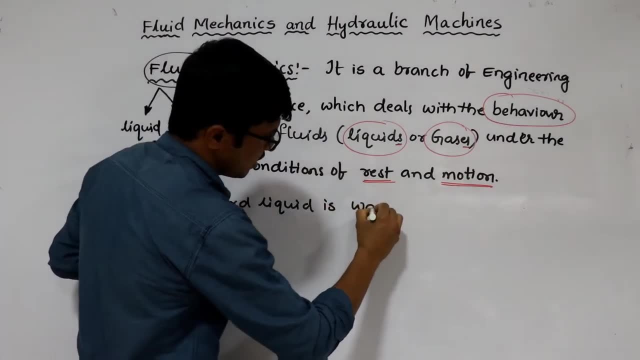 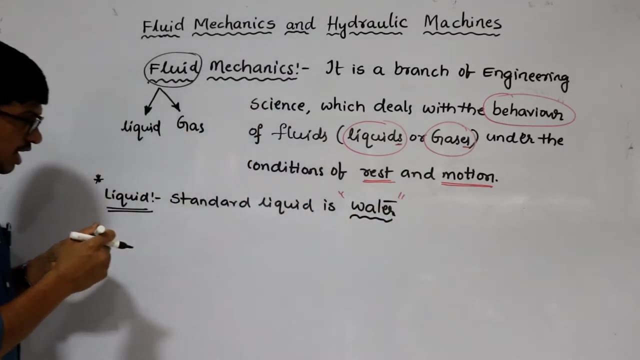 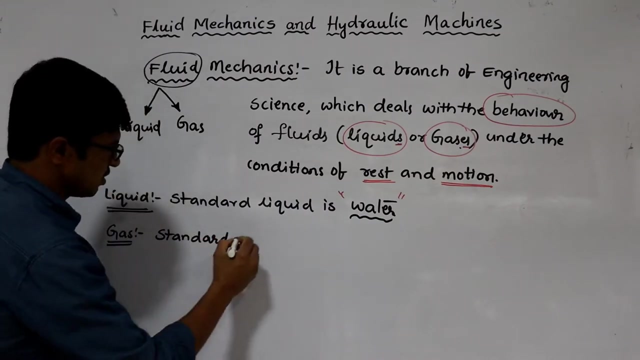 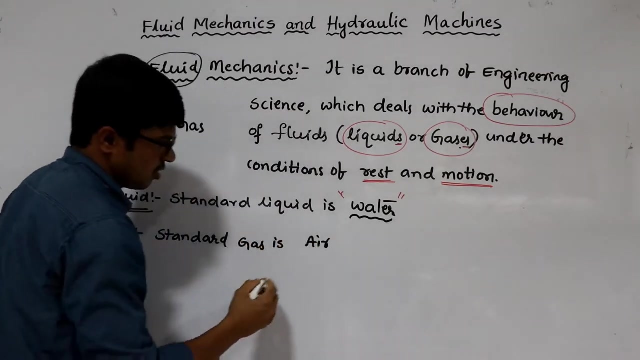 So the liquid standard liquid is standard, liquid liquid is water, Standard liquid is water, And similarly we have gas here, gases. So in gas the standard gas is Standard, gas is air, standard gas is air. 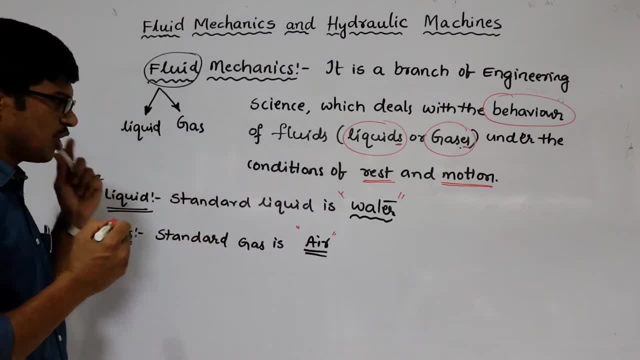 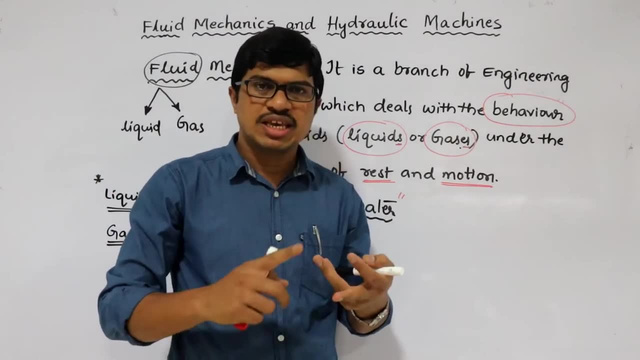 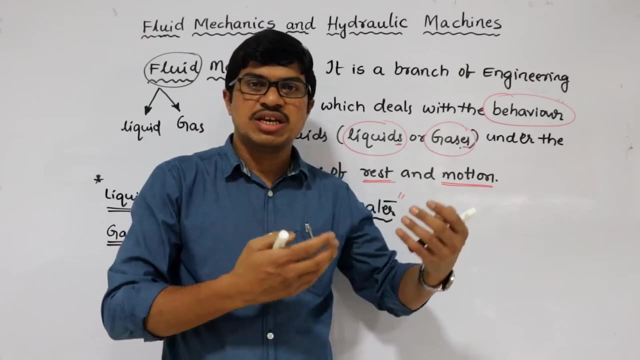 So these two points are very, very important. and another important point: the liquids either. let us consider- I think every one of you are aware about- the petrol, diesel, kerosene liquids, which are the liquids right, and other than that also, especially in kitchen itself, you. 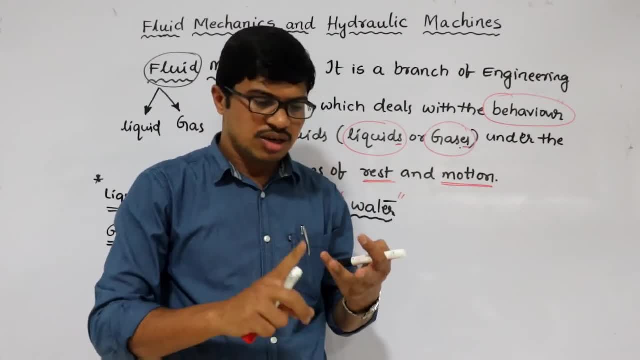 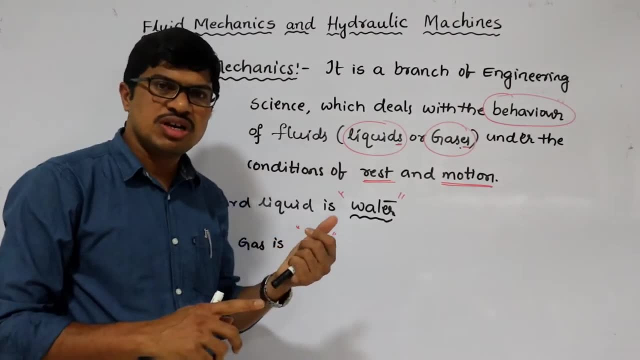 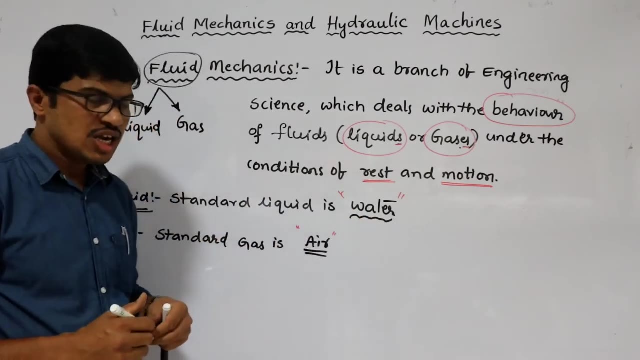 can find oils, right, curd, honey, which are also comes under liquids only. but when it comes to gas, LPG, CNG, which are all comes under gases, but standard liquid is only water and standard gas is only air, So the liquids always, which are incompressible. we cannot compress the liquids. 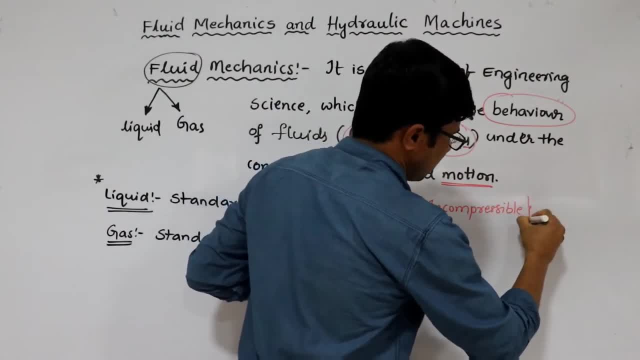 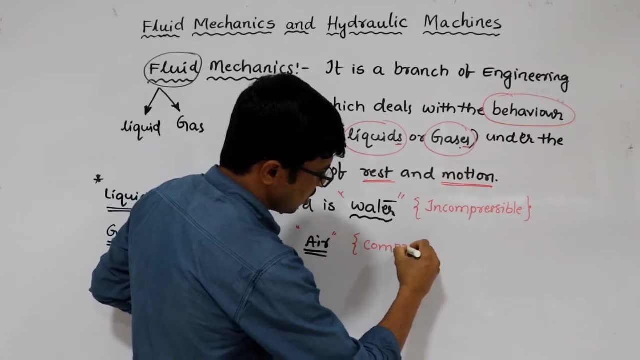 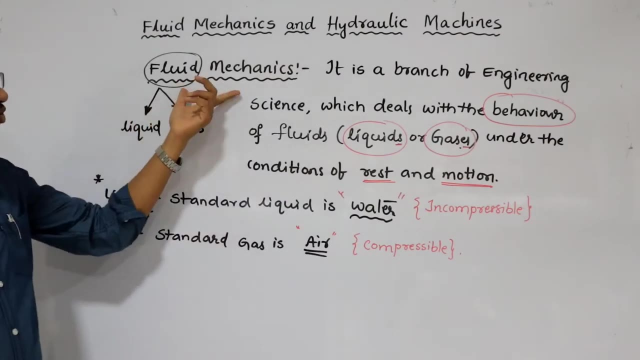 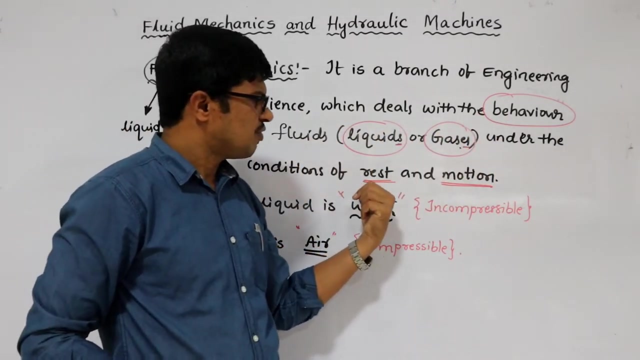 Liquids always incompressible, but gases are compressible. gases are compressible. So I repeat again, the fluid mechanics: it is the branch of engineering science which deals with the behaviour of the fluids under the conditions of rest and motion. So then, after we will see what is fluid rest, 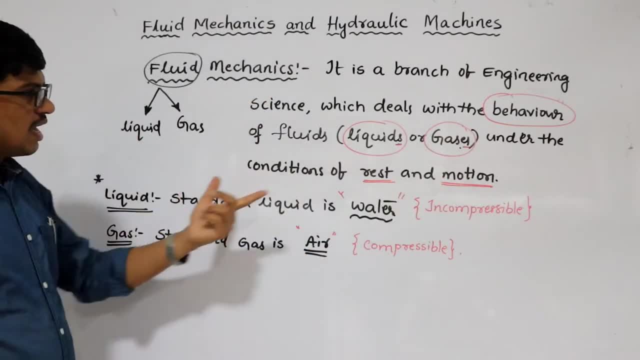 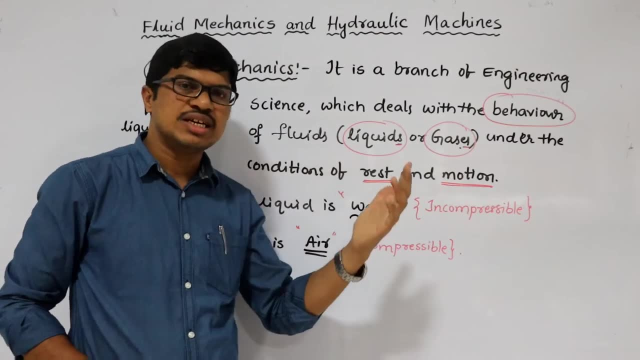 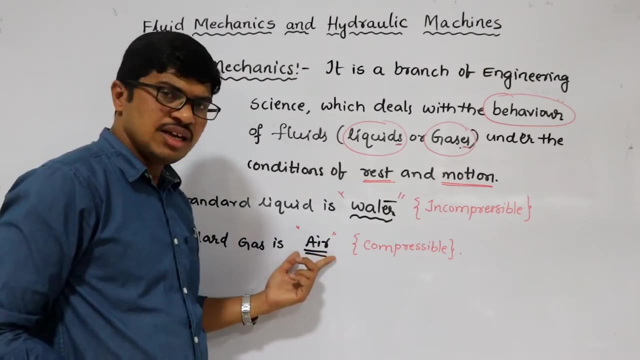 And what is fluid is in motion and here, as I mentioned here, liquids and gases. the standard liquid is water and the liquids, not only water, the other than that, whichever the liquids, which are all incompressible, only the standard gas is air and other than air. we have many, but 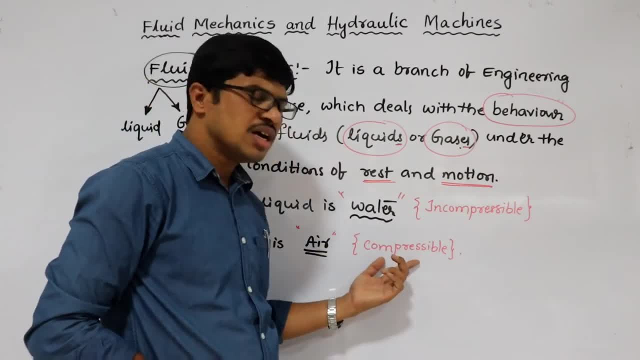 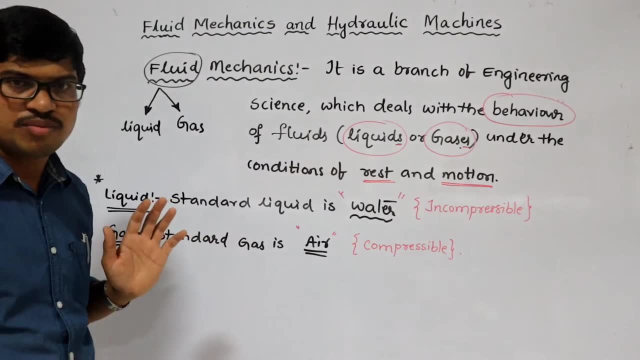 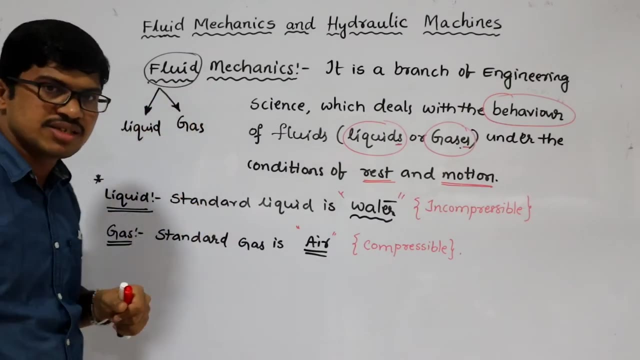 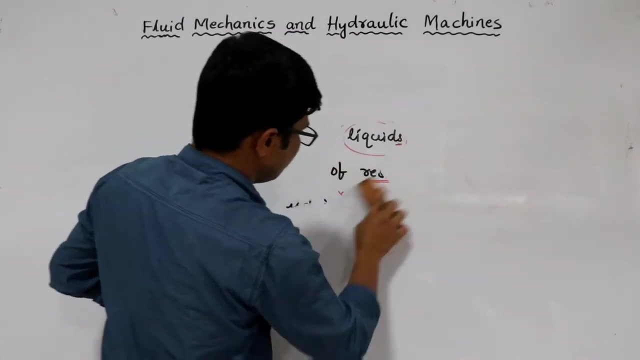 not standard right like LPG, CNG, then everything will comes under compressible only. So gas is always compressible and liquids always incompressible. So these are very important points right Now. after this, let us see what are the classification of fluid mechanics. 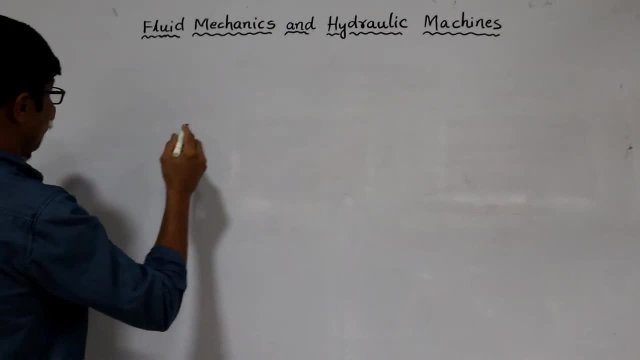 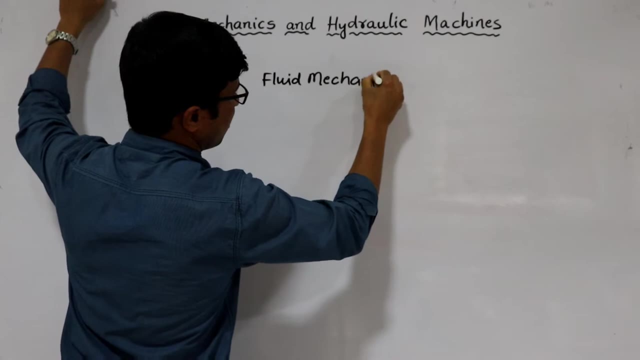 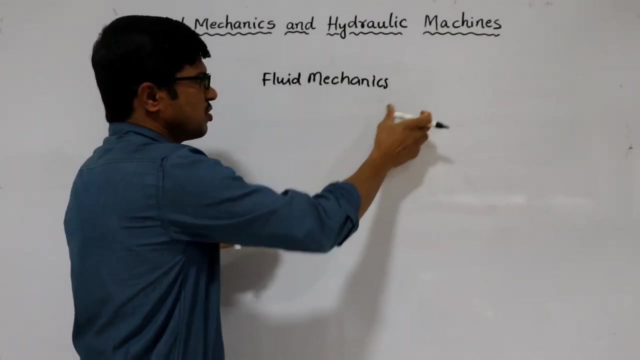 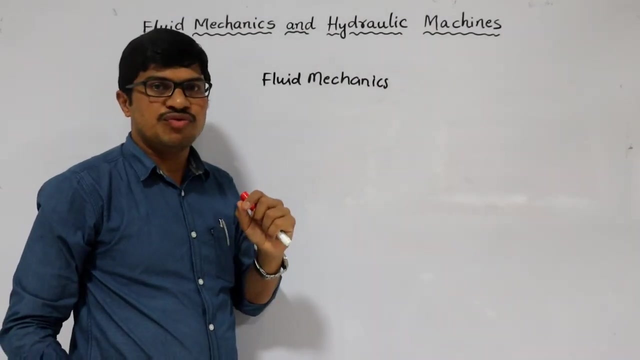 Now here, fluid mechanics, Fluid mechanics, Fluid mechanics. So generally you might have seen in many textbooks which are classified into two types: fluid statics and fluid dynamics. but as per my way of teaching I will do small correction here, but definitely this method also, it is correct. 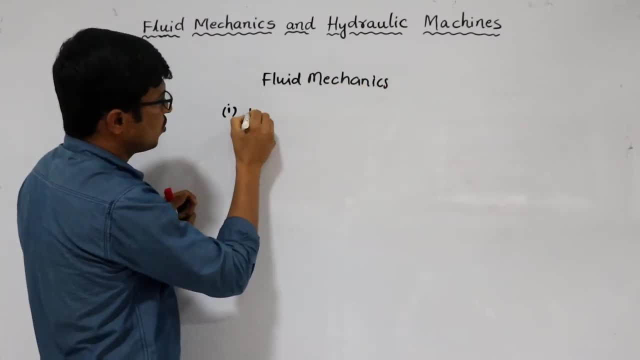 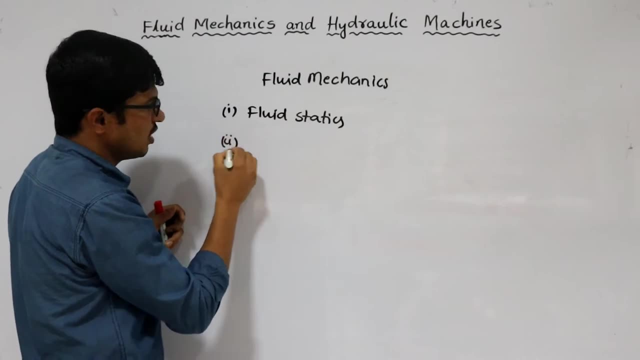 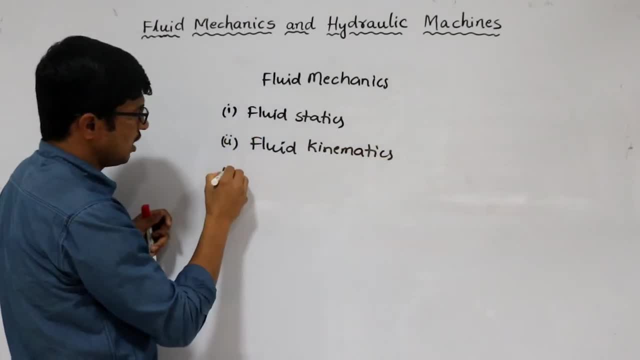 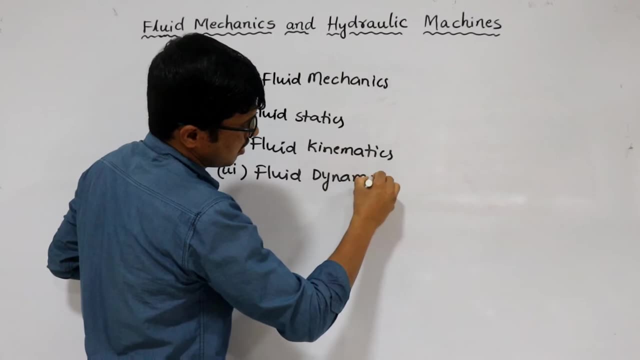 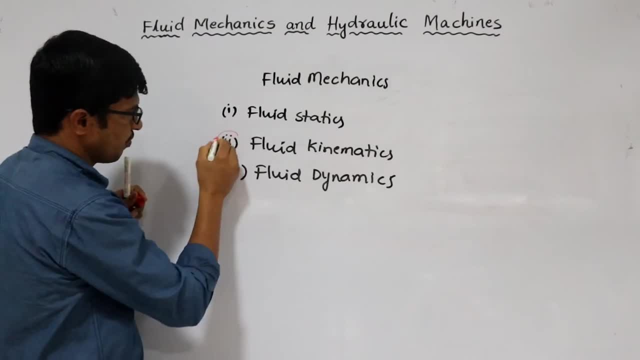 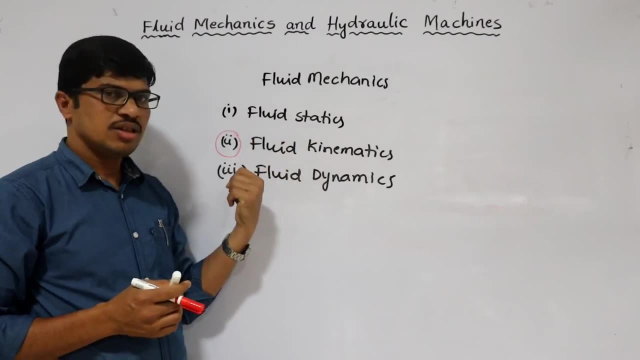 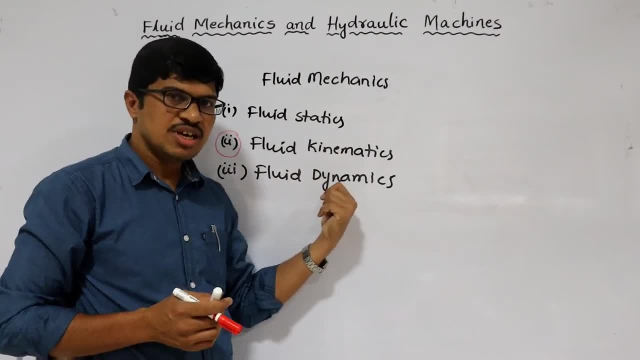 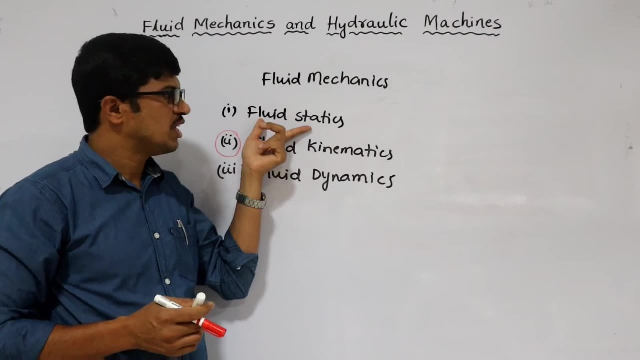 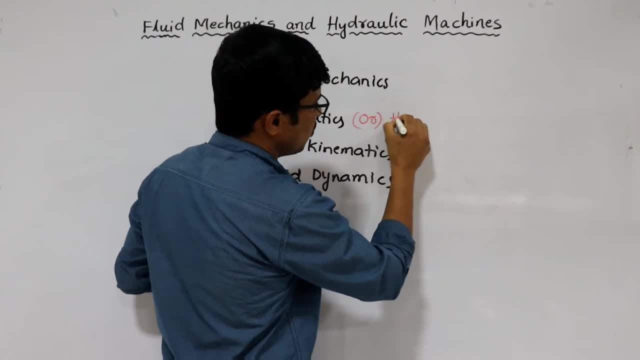 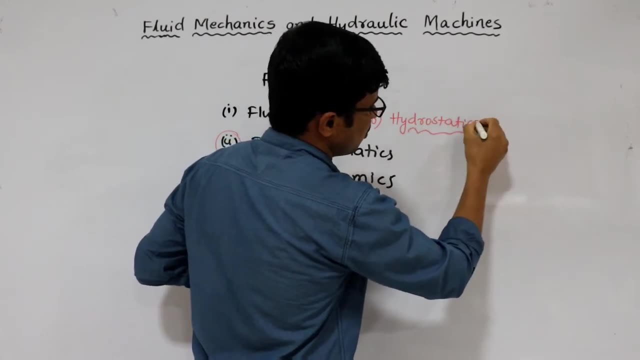 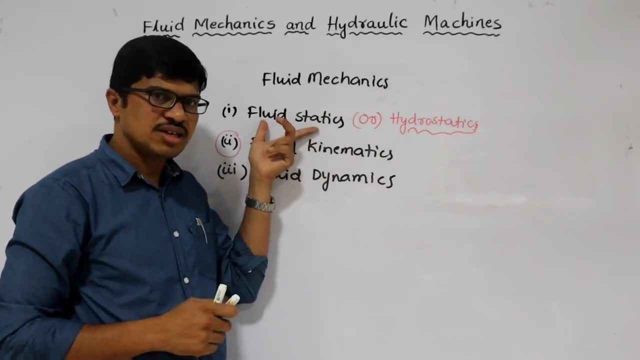 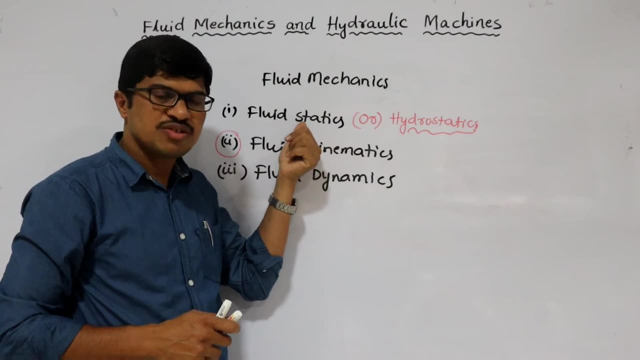 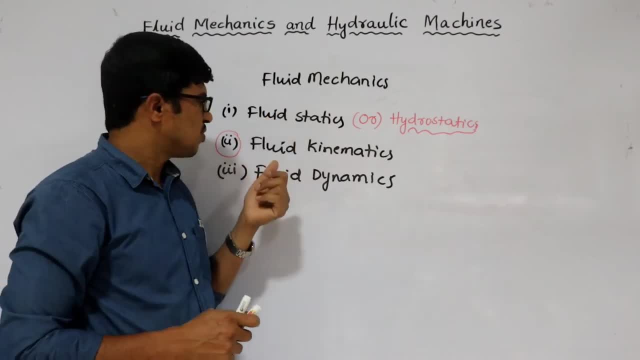 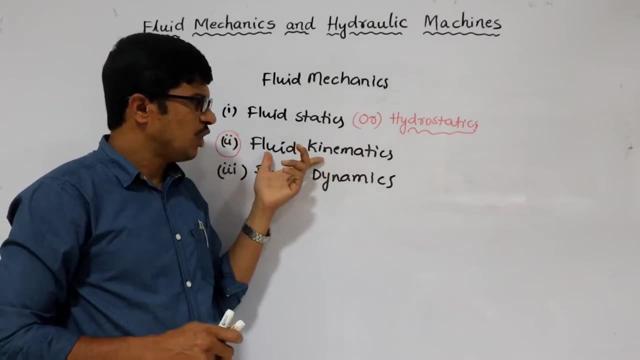 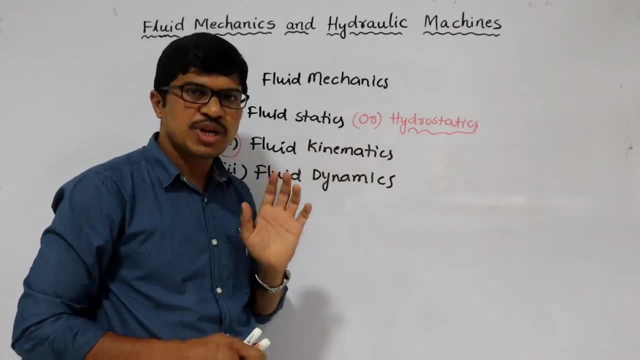 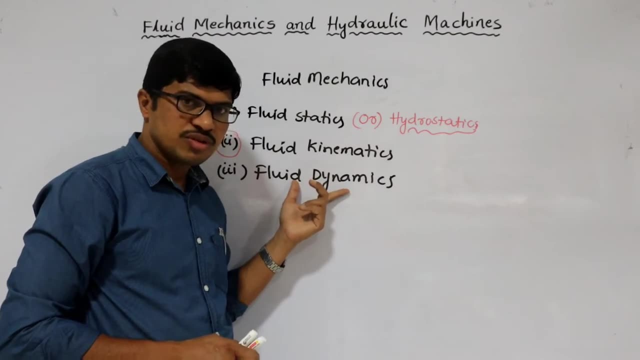 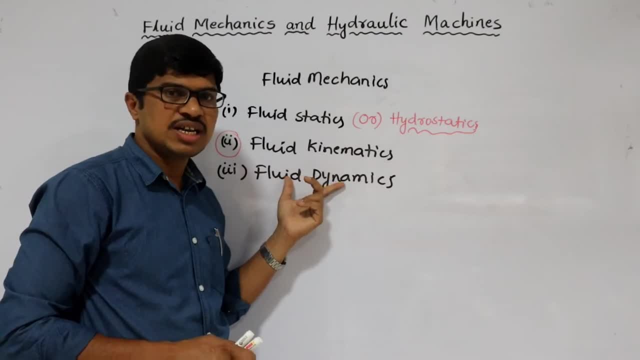 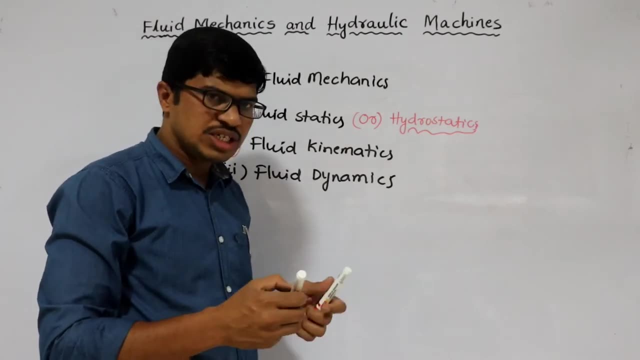 Pressure forces are considering- Pressure forces are considering. That is called Fluid dynamics. Now you see one by one. now, Right, And according to JTUH for Mechanical, The syllabus is- This is lesson number 1.. This one is- This one is Unit- Membership Test. 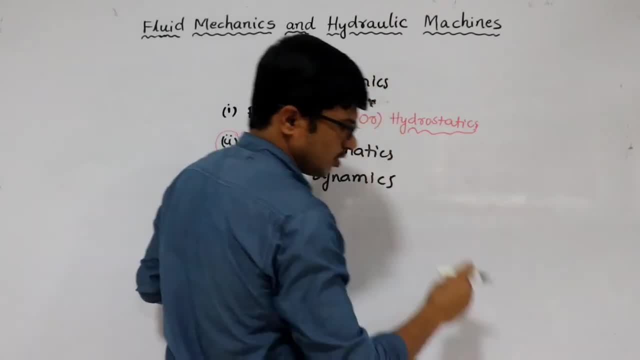 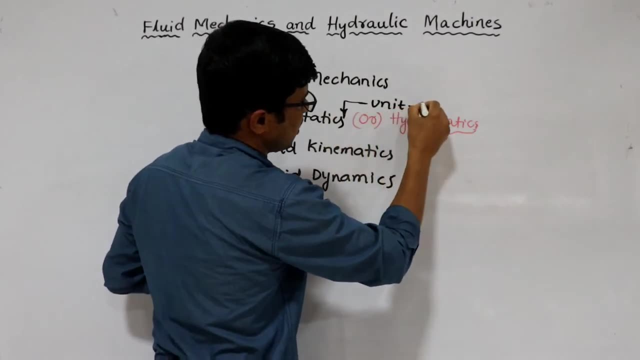 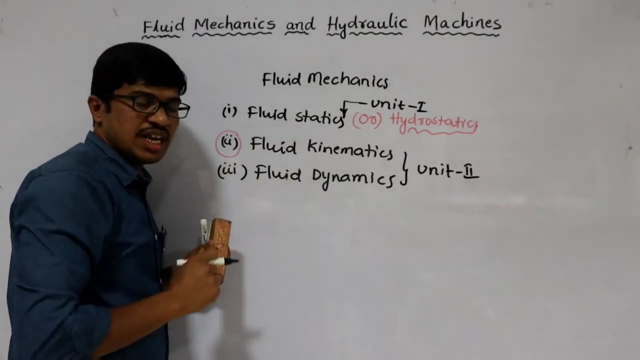 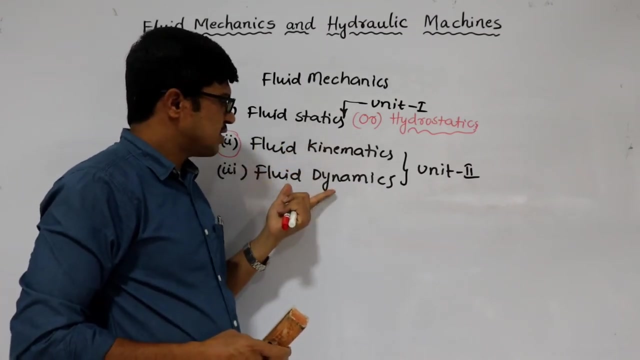 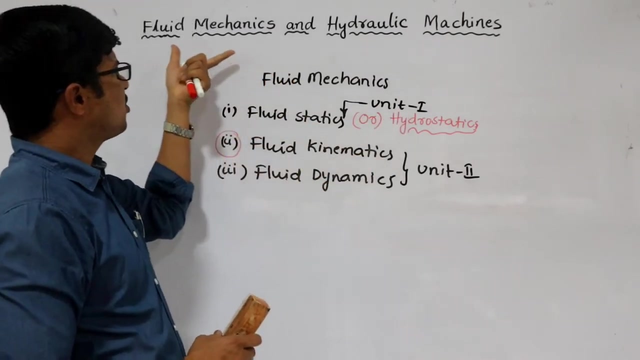 Okay, Okay, Now we know- guys. Now in these ح, x, y equations 1 and these two are unit 2 for mechanical students, right? so first i will give the definition of fluid statics and fluid kinematics and fluid dynamics, then after that i will start. what is fluid statics? that is lesson number 1, right, and this introduction part also will come in the lesson number 1. only, what is fluid mechanics? just now i have given the definition. 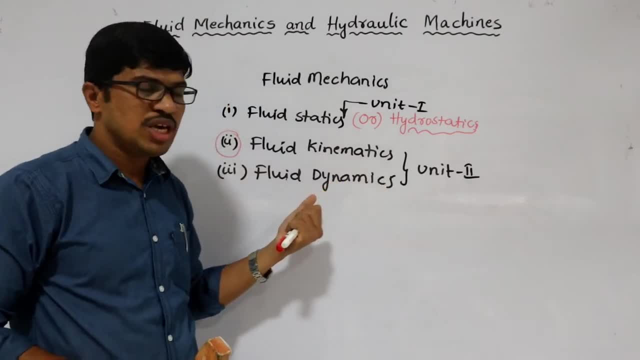 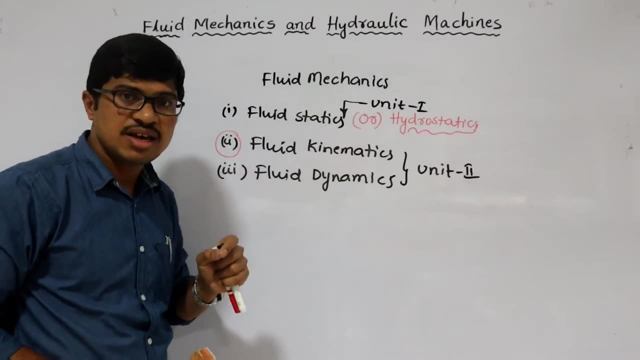 the fluid mechanics. it is a branch of engineering science which deals with the behavior of the fluids addressed as well as in motions. right and standard liquid is water and standard gas is air. please remember, this is very, very important right now. let us see. the first one is fluid statics. 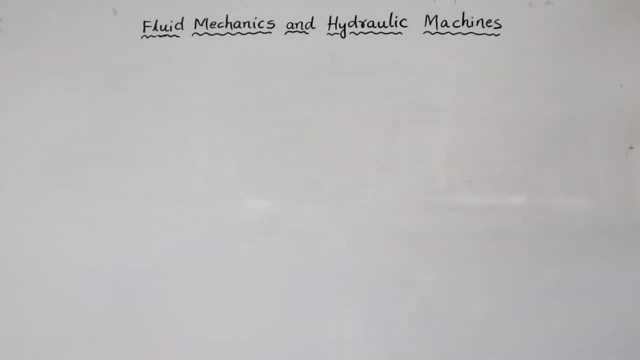 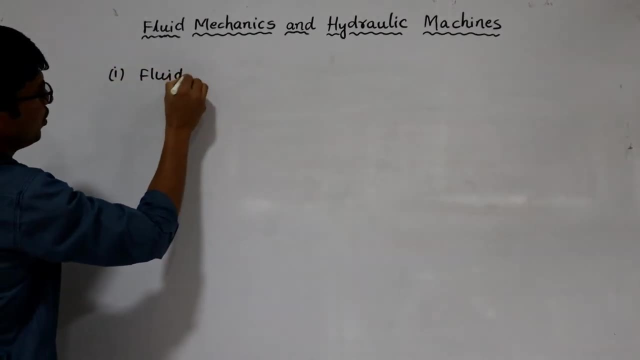 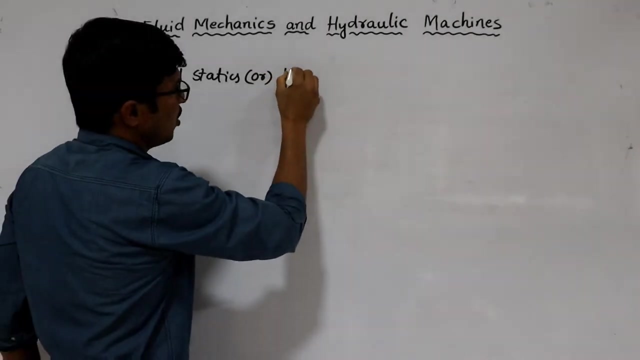 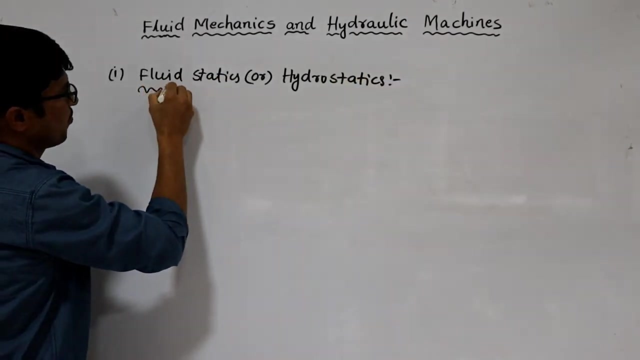 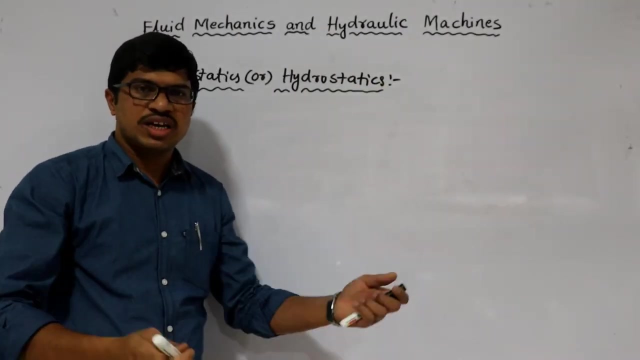 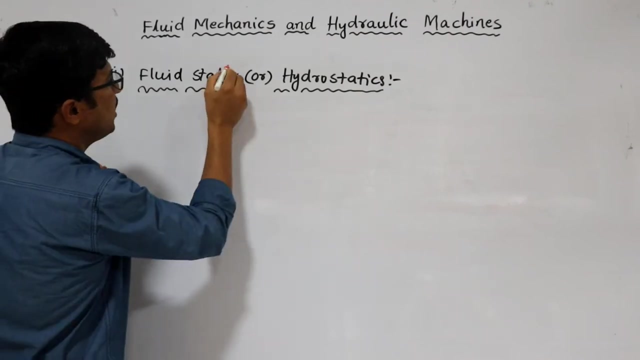 that is also called first one is fluid static or it has another name: hydrostatics- hydrostatics. so very simple, i think, do not require more technical knowledge here. easily you can understand the fluid static. so we need to have a basic knowledge what you mean, the meaning of static. 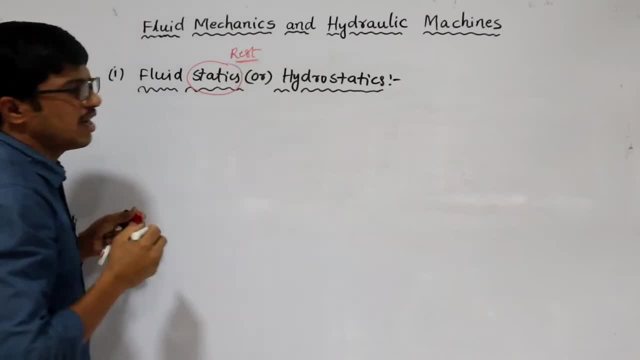 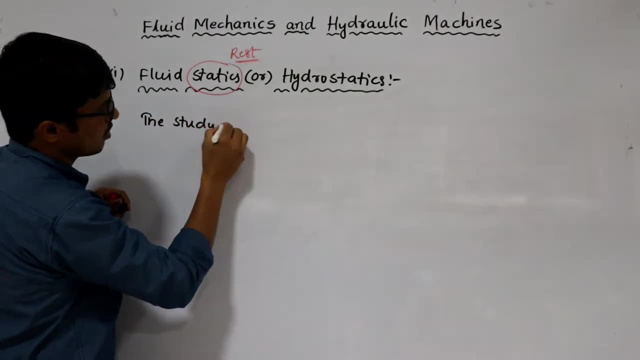 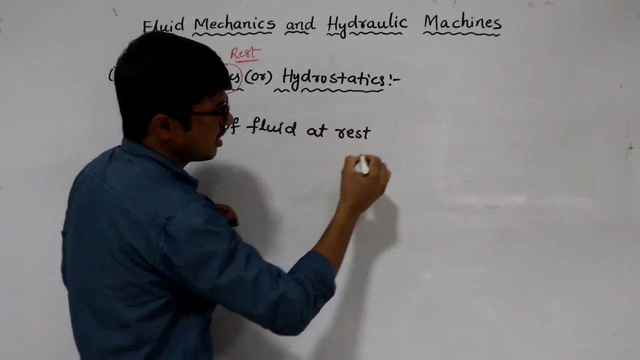 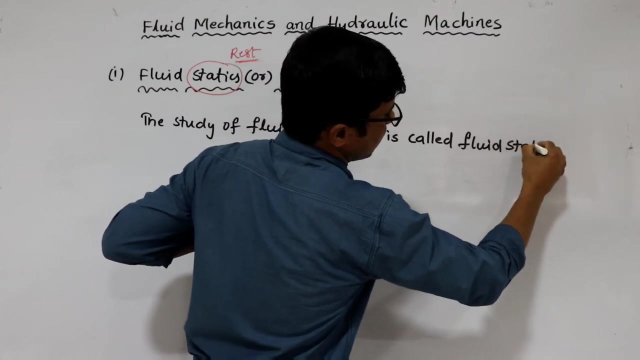 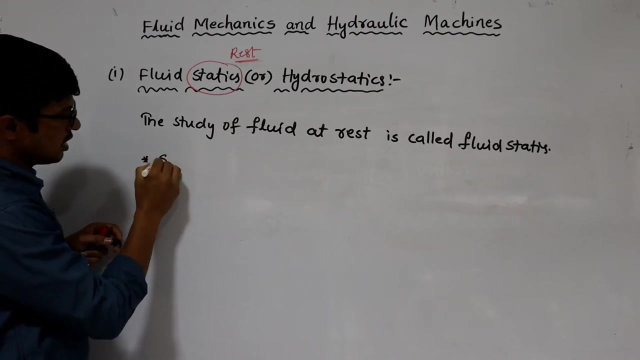 static is nothing but rest. static is nothing but rest. static is nothing but rest. so here, look at the definition of the study, of the study of fluid at at rest is called: is called fluid statics. is called fluid statics and, very important point, here the reading is: 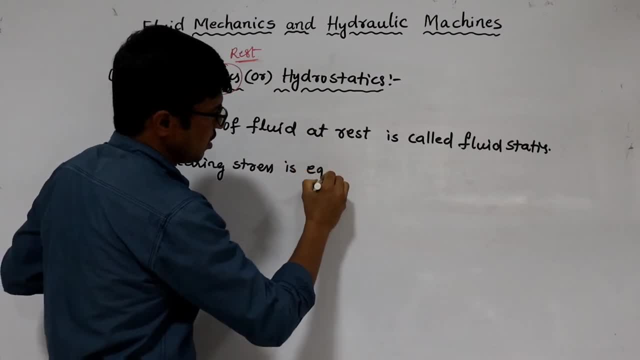 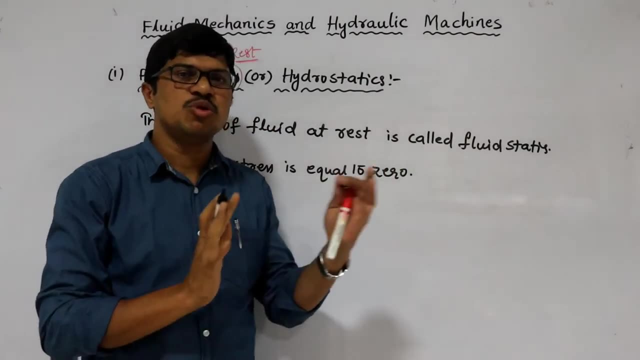 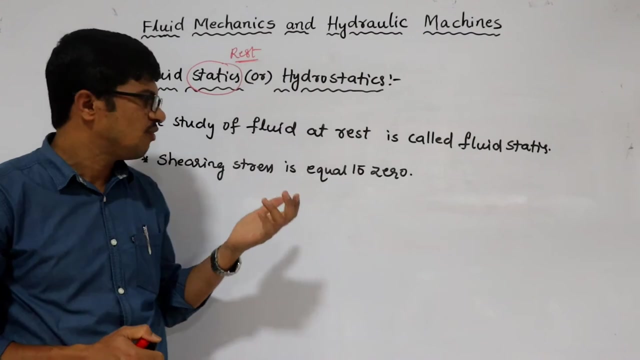 a Esther shearing stresses equal to the floor because it does not have any motion here. very good, because they're the cause of work when the functional forces are acting or the fluid, so definitely we can say that and then we strongly share: these places are producing. but here in this particular complementary, the Watson already, which is at rest, the means what the velocity is equal to zero, and then definitely study that as well. you have, show you 30 if you learn a new aspect, correct after operating theory, possible internal difficulties, that is that we cite the freezer yourself. here you go and you will get especially very Smith to be good, or nor does a full, and can change a little that here. now there is something there. you haveحم politist learned that it is it. 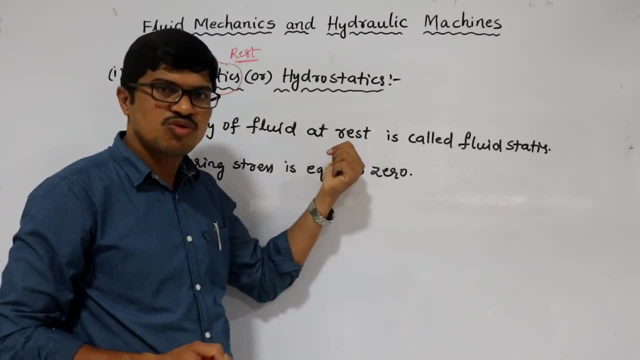 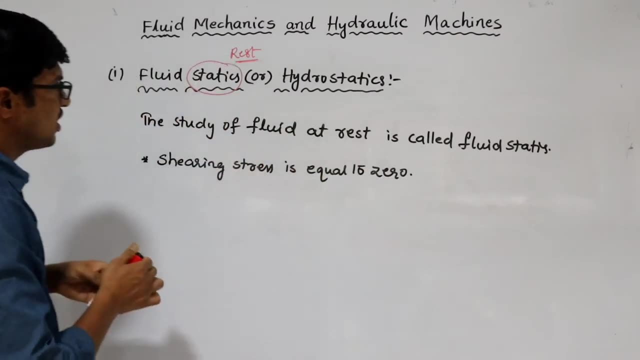 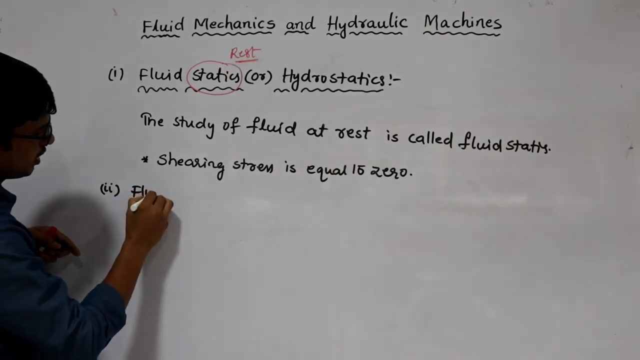 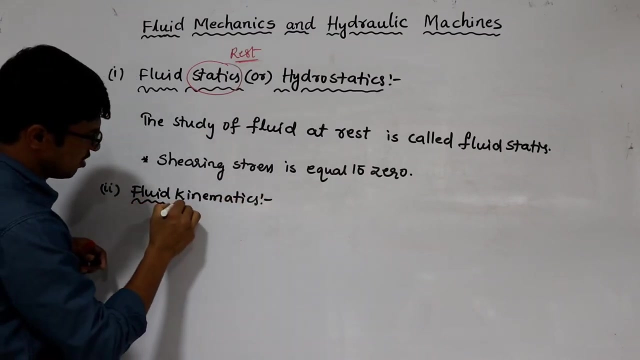 you test these global question ofmetrics. you know the 부 of today. the velocity is equal to the stress level. you know its level. you know what is equal to the stress level, gia, So definitely we will get shearing stress also equal to zero right Now. next one is second one: Fluid kinematics. Fluid kinematics- It is also very easy, So let me write the definition here. 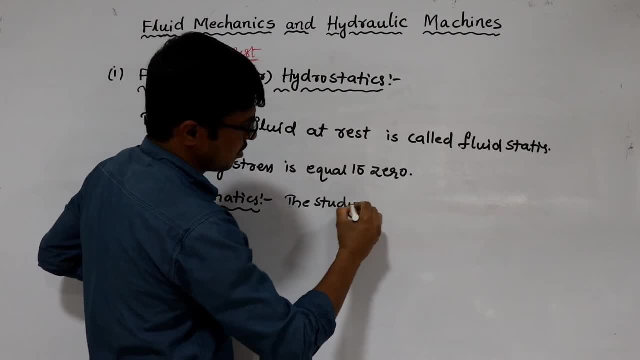 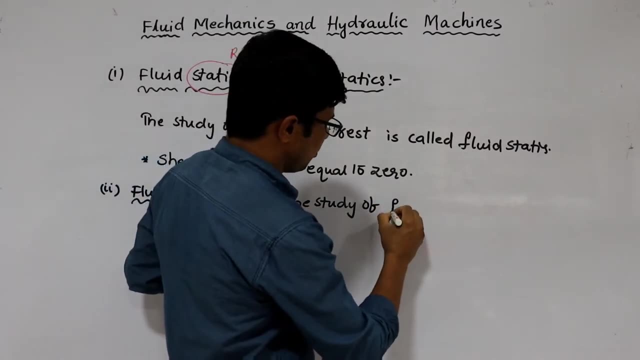 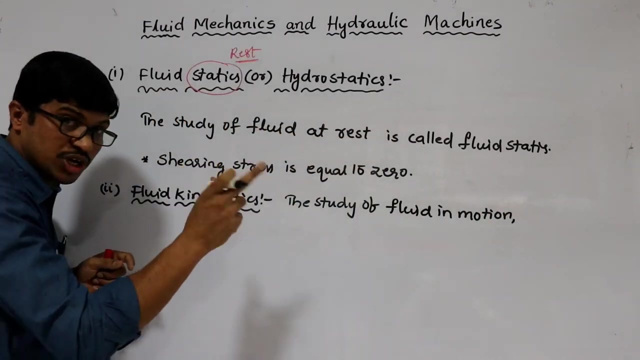 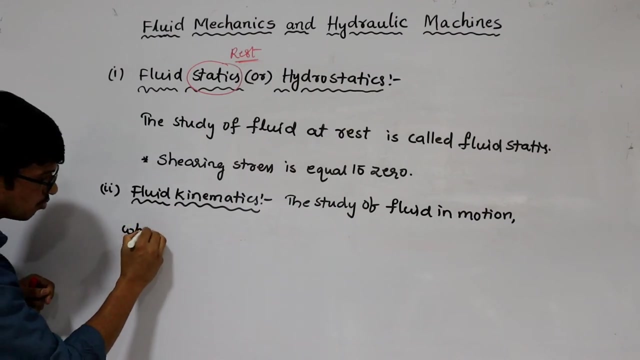 The study of, The study of, Because generally we know kinematics is nothing, but we will be having some velocity right. So the study of fluid in motion, In motion, But- very important note, Still it is not completed. The study of fluid in motion where- this is very important point- Where pressure forces are. 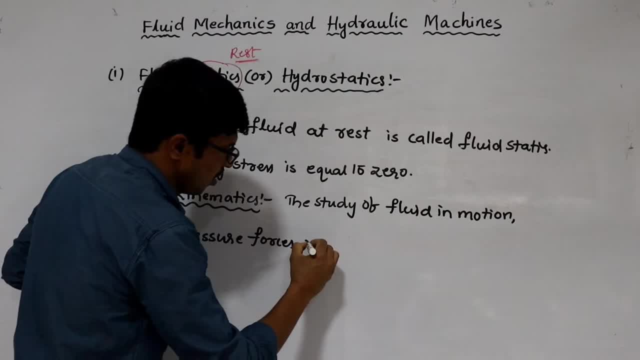 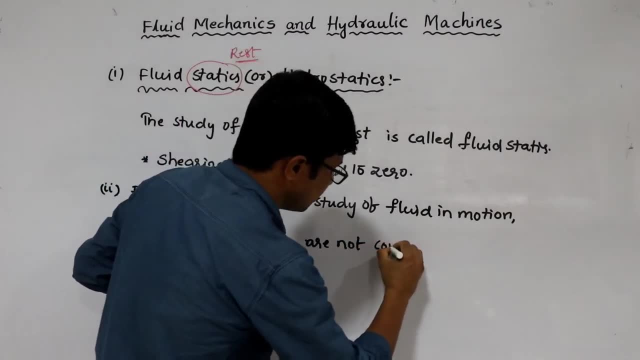 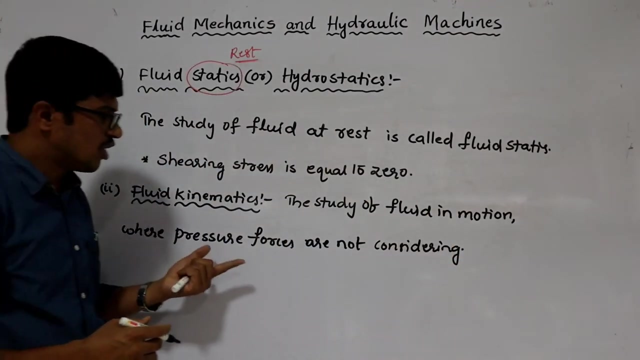 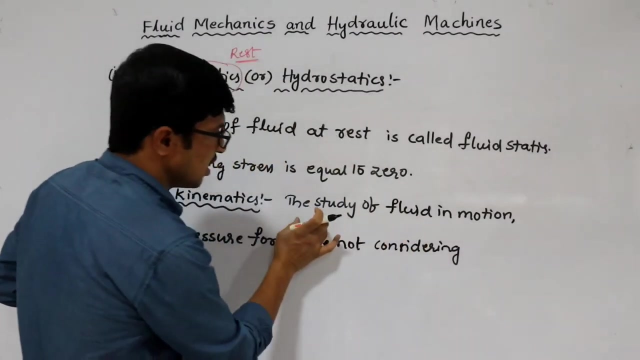 Pressure forces are not considering, Pressure forces are not considering. So without pressure forces the study of fluid in motion is called fluid kinematics. So we can write here: The study of fluid in motion where pressure forces are not considered is called fluid kinematics. 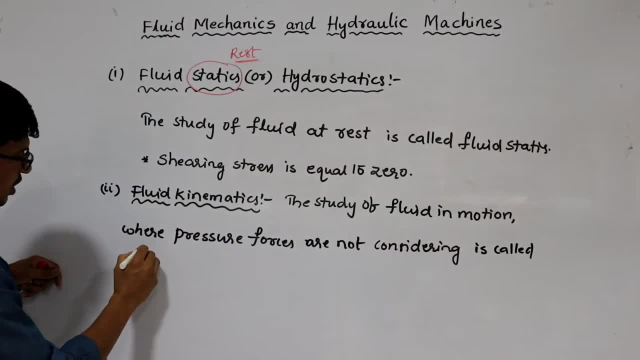 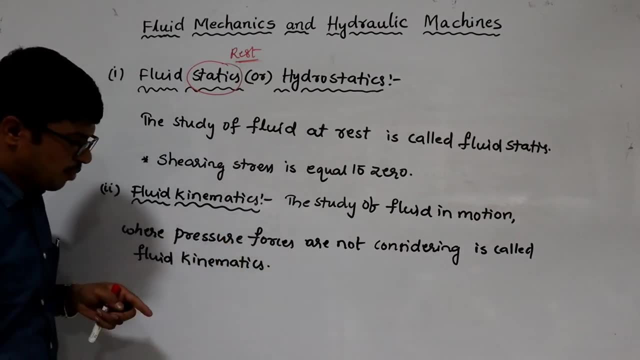 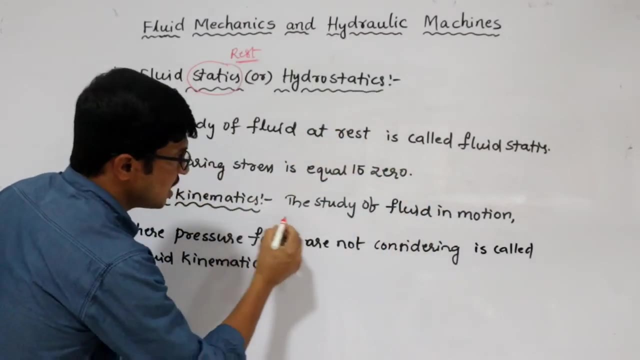 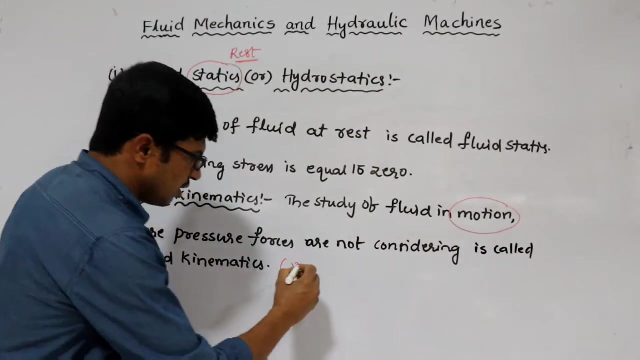 Is called fluid kinematics. It is called fluid kinematics, Fluid kinematics, But here you can see the velocity will be there. That is a very important point. Here we are considering motion. So definitely velocities will be there And definitely there will be a gravitational force, right? 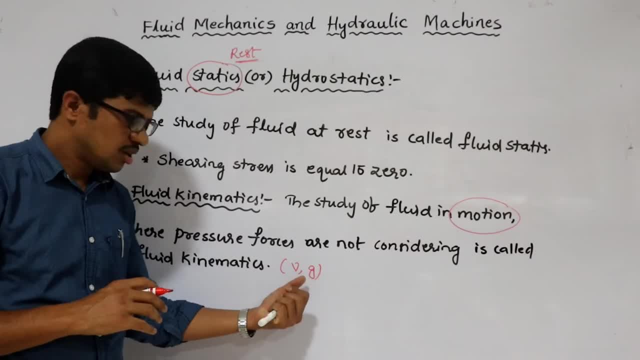 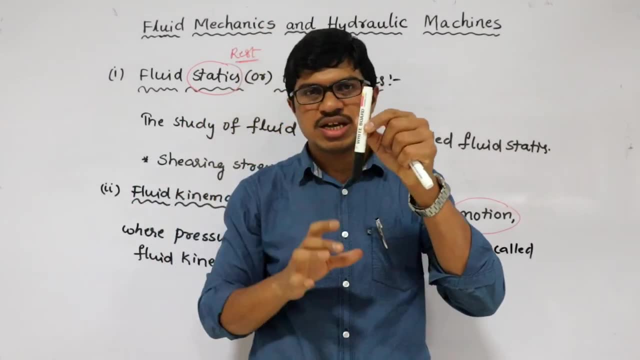 Gravitational force Right Gravitational force, Gravitational force, Gravitational force will be there and velocity will be there. let us take now. i have some object here, so it is a solid right. but let us assume i am having some glass of water once if i start bending, so definitely. 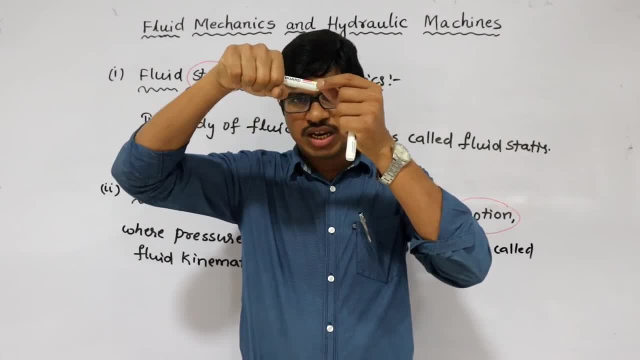 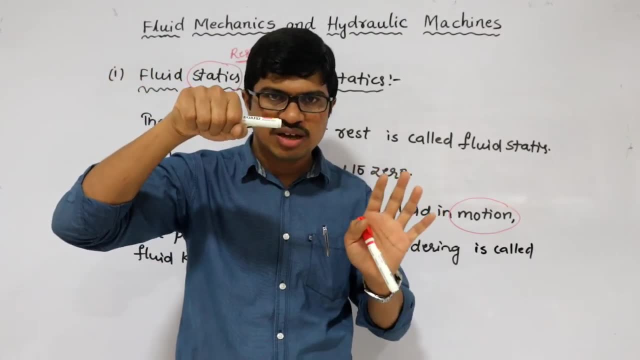 the water will start falling down. so water which is falling, it's due to gravitational force. so gravity, i have considered here. am i applying any pressure here? no pressure forces are acting, simply the water which is, freely, it is falling down. so that means what the water which is having 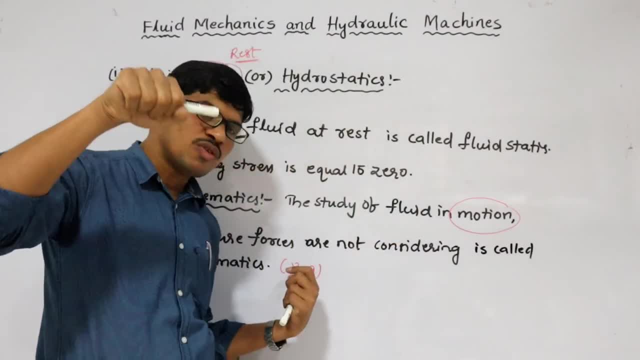 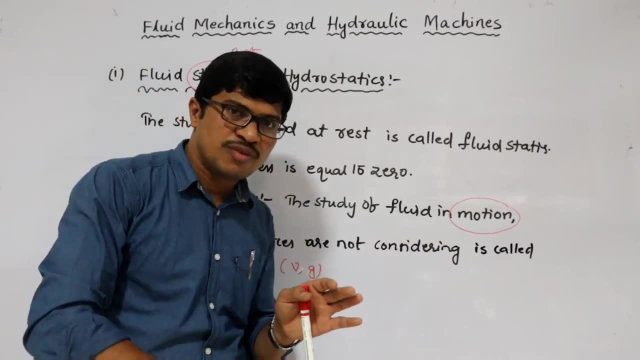 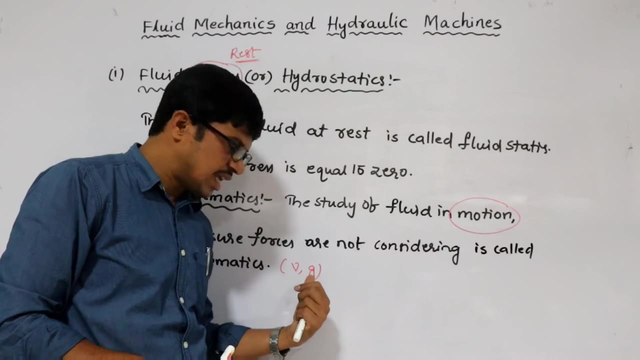 some velocity, so velocity also, i have considered. so water will be having no, no pressure force, but velocity, because it is flowing right, and here it is not possible from low level to high level, it is only possible from high level to low level, from high to low. velocity and gravity will be. 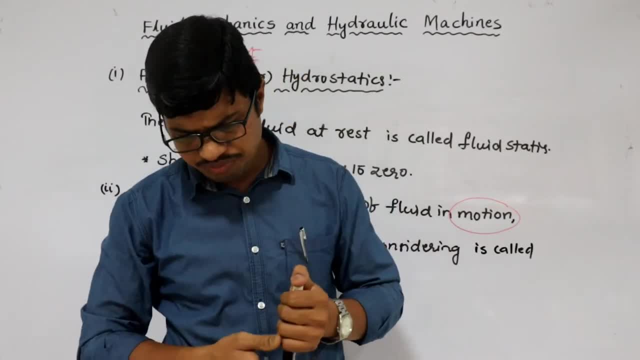 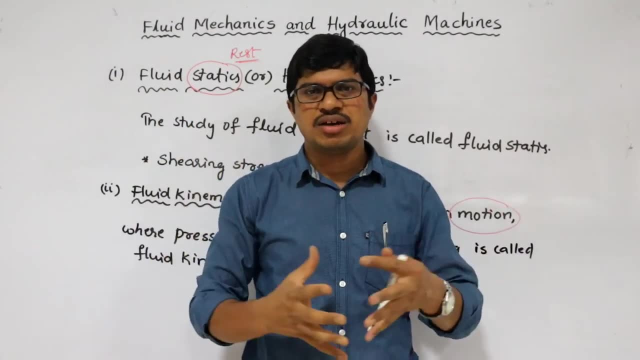 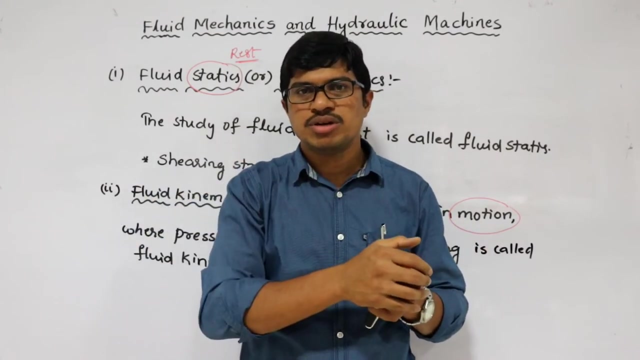 occurs. and one more important thing let us consider entirely. we can see also, especially in house. suppose in fourth floor there is a some tank right from some to. we are filling the tank, but while in kitchen cleaning something right, we will open the tap. is it required any specific motor to pump the water from higher to lower? that is called a kitchen. 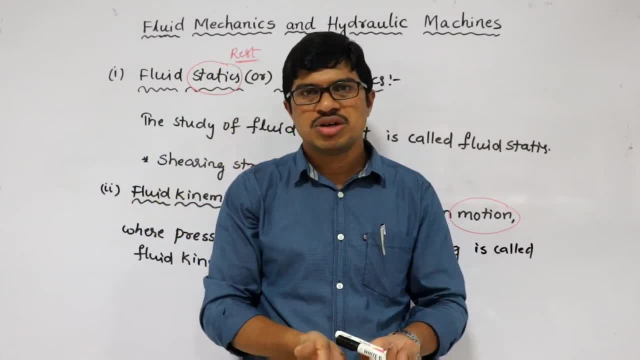 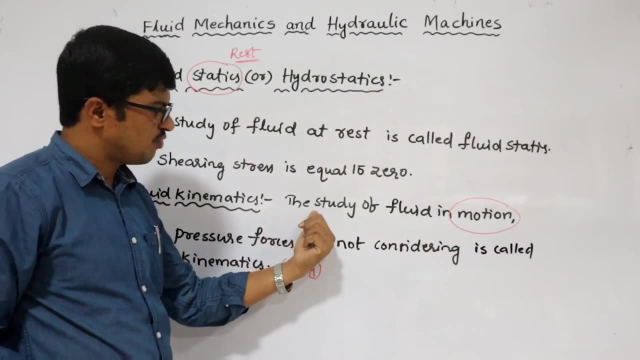 not required. just simply you need to open the tap. that's it, it will come out. so that is under kinematics only. it is not under dynamics, clear. so as simple as, but you can have a definition here. the study of fluid in motion where pressure forces are not considered is called fluid. 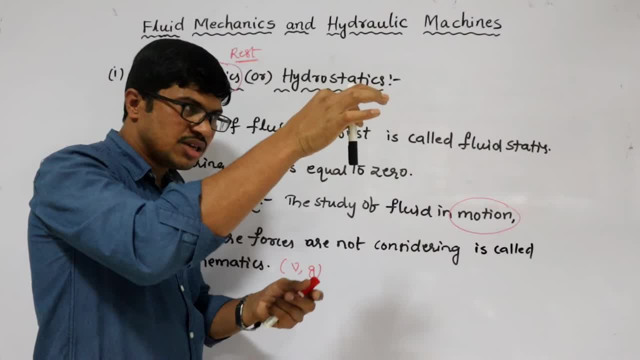 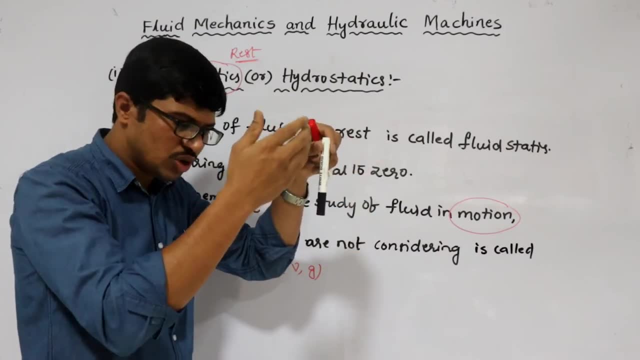 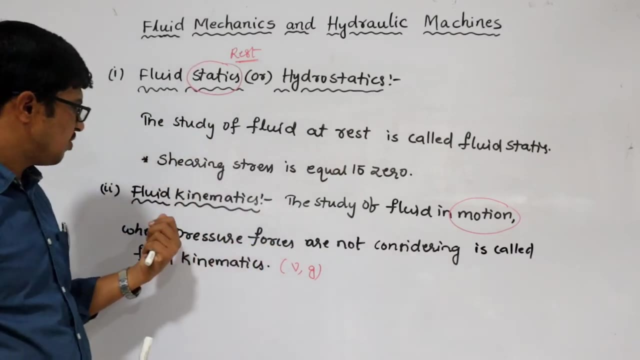 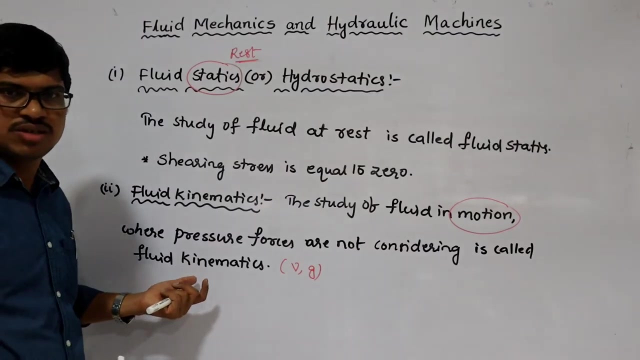 kinematics. so very simple definition. just, if i release this particular object, it will start falling down. so here i am. i am not applying any force due to gravity. it is falling down and while falling will be having some velocity, so velocity and gravity will be there. and especially here we study about translation, rotation and deformation of the fluid elements. 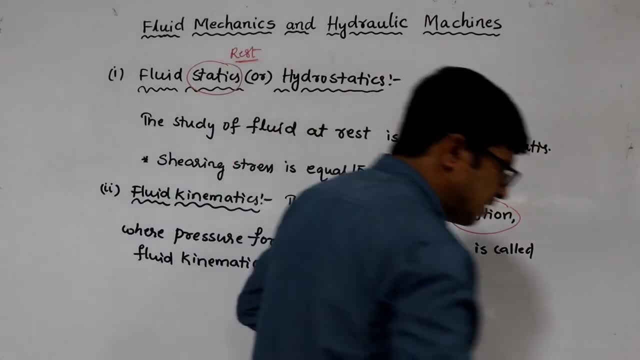 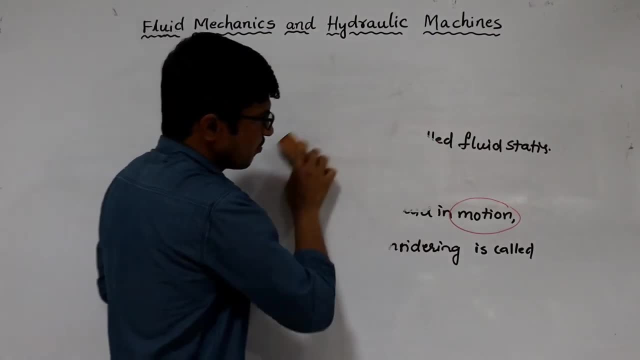 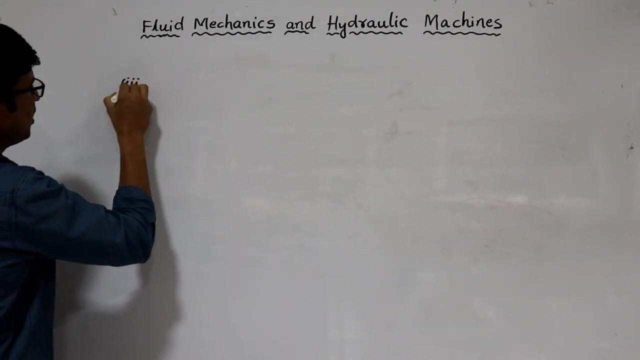 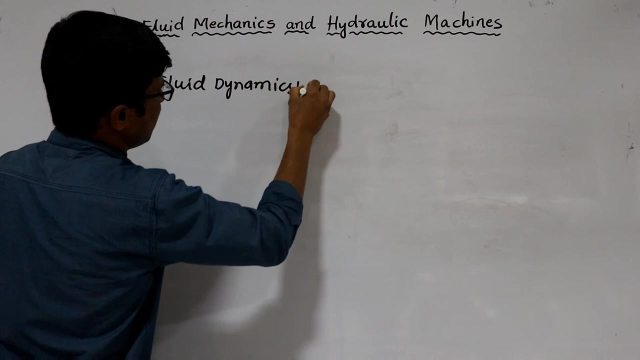 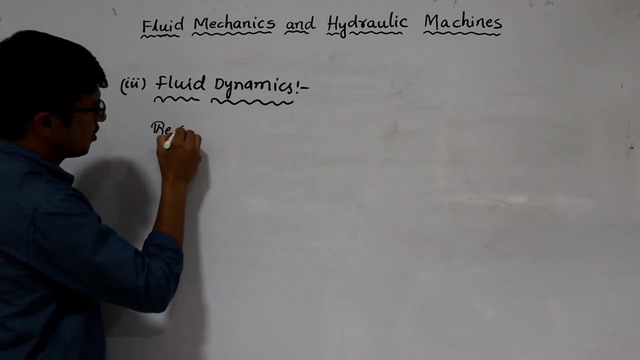 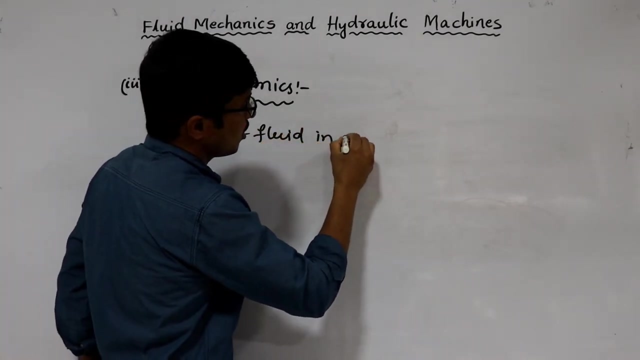 clear. that is about the fluid kinematics. so let us see the third one: fluid dynamics. the third one is fluid dynamics. so in dynamics you need to consider the pressure forces. third one is fluid fluid dynamics. so very simple again here: the study of the study of fluid dynamics. the third one is fluid in motion. for kinematics and dynamics it is common here till here. 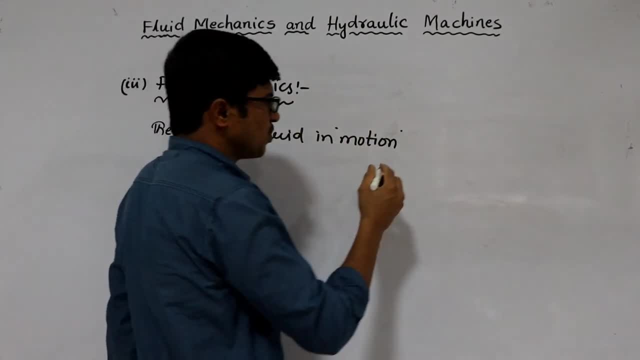 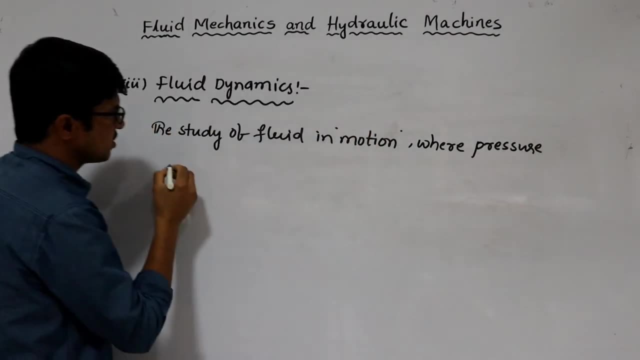 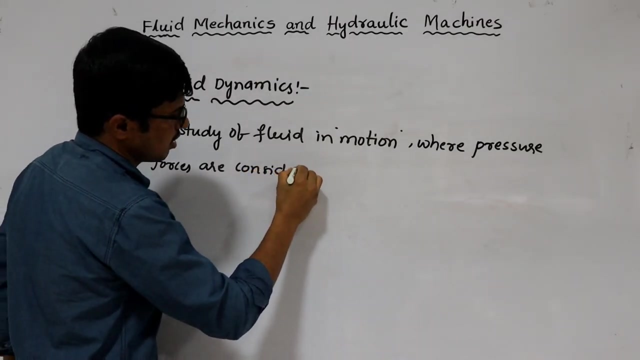 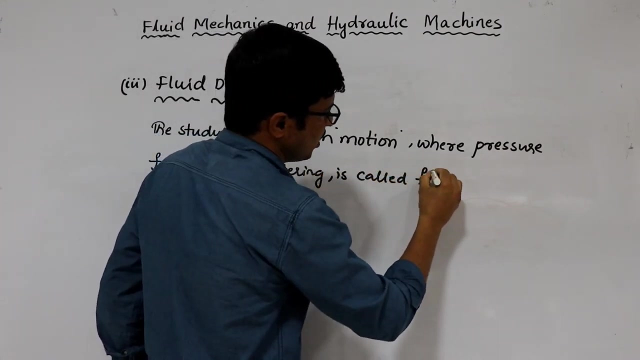 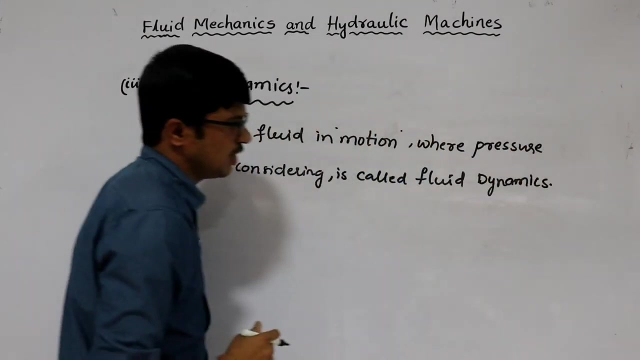 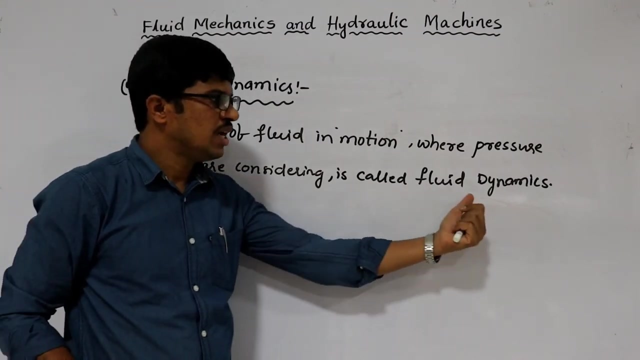 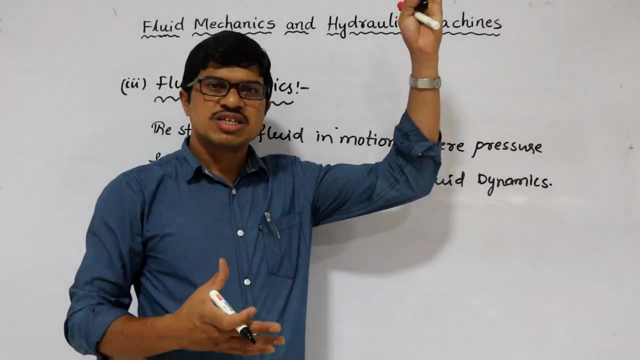 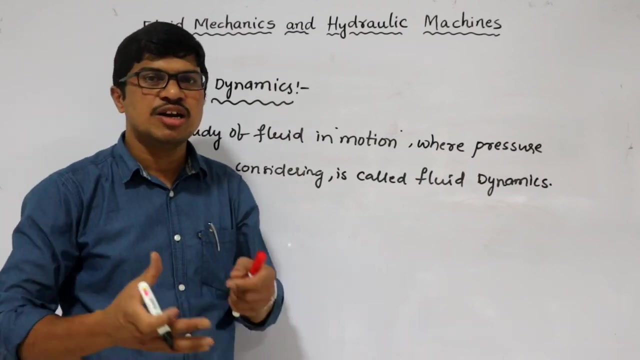 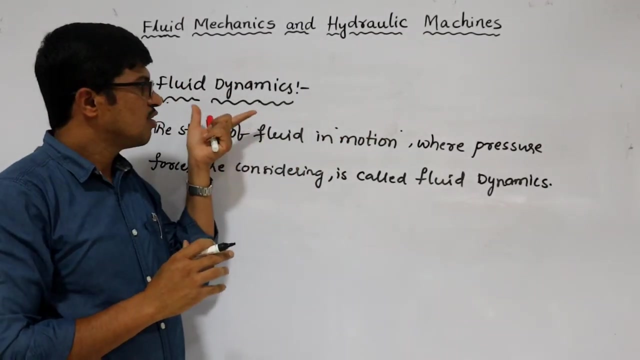 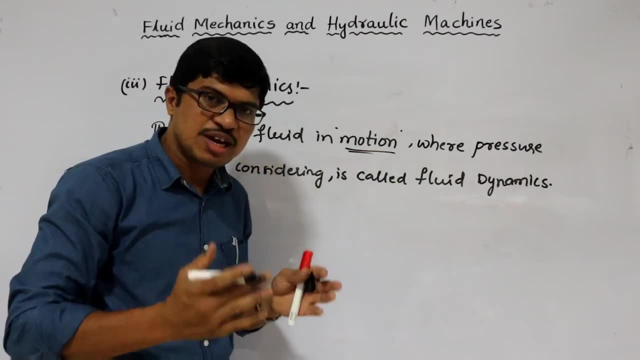 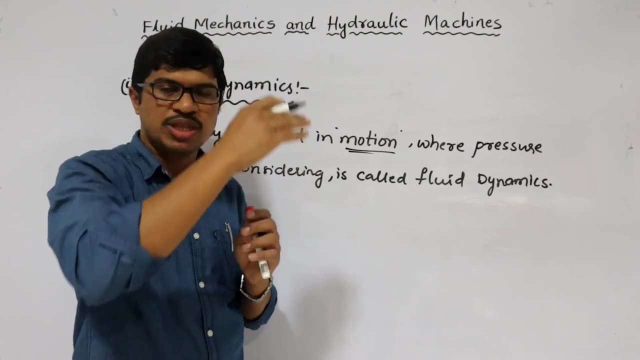 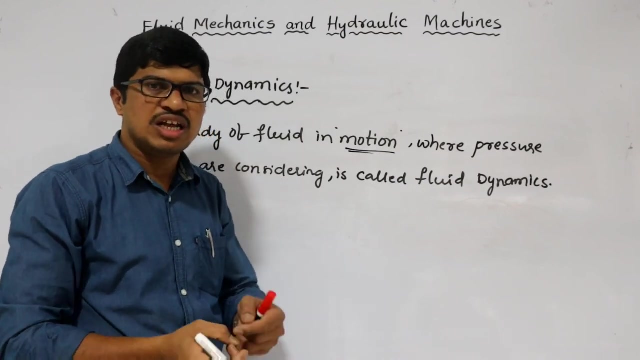 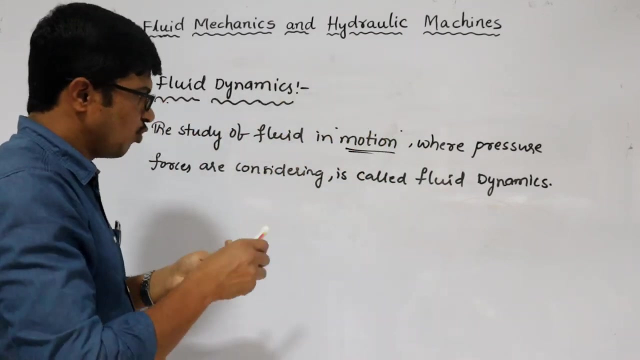